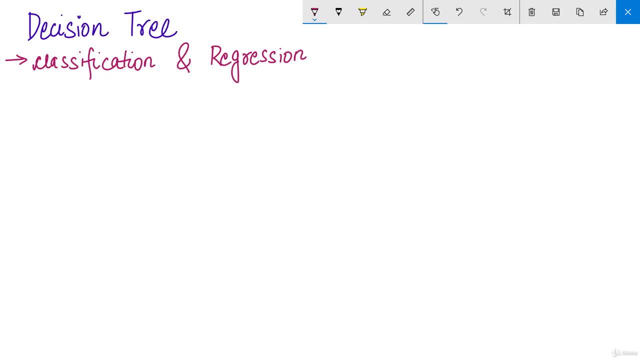 go through the classification integration concept once. all right. so, like in daily life, we take, we do and we take decisions right. so in decision analysis, a decision tree can be used to visually and explicitly represent decision, and it helps in decision making as well. so, as the name suggests, as the 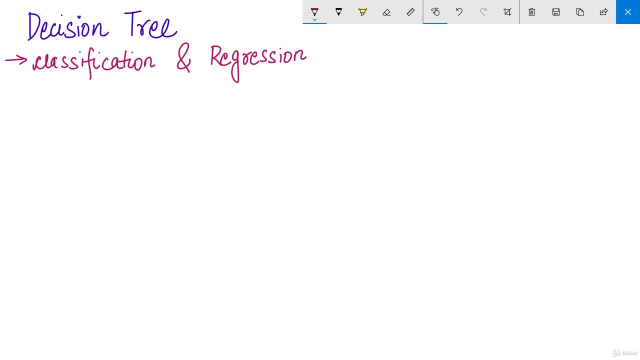 name goes it is, it uses a tree like model of decision. so I just note down the important points: tree like model, okay. so like it is widely used in machine learning, like in basically your machine learning, which will be our main focus, but let me also tell you that a 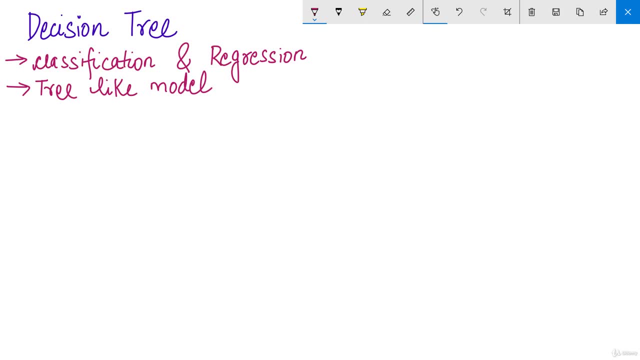 the decision tree. the tool which is used is commonly used in data mining and where it is like those who are from data mining background, they must have, like they must have a good understanding of decision tree, where they must be using it to derive a strategy to reach a particular goal, like, whatever the 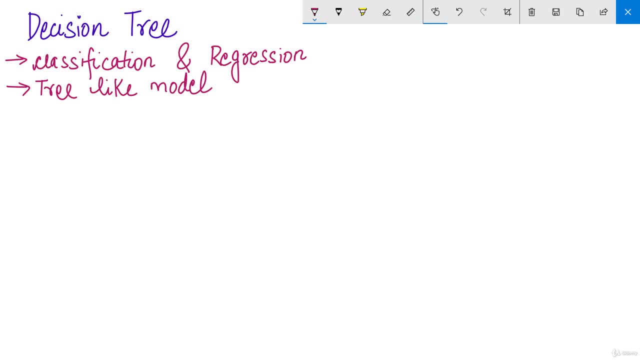 strategy they use to reach a target like this: make a target and how to reach that target. they use decision tree concept there, as well in data mining. so in machine learning it is also important and as well as in data mining it is widely used. all right, so like: how can an algorithm be represented as a tree? 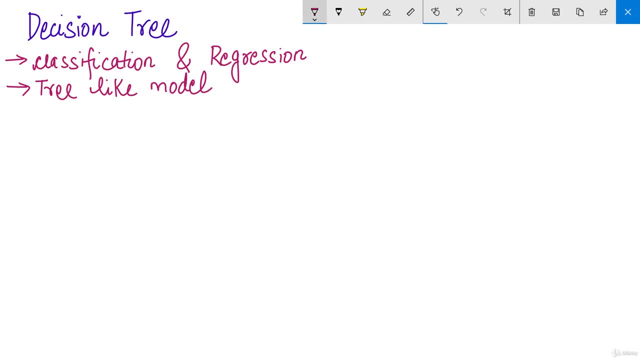 so let me explain you by giving an example. suppose let's say there is a patient- okay, so this is a patient- and and he went to a doctor and he said: that doctor, I have a chest pain. let's say he said chest pain, he has having a chest pain. so what doctor will say what doctor? 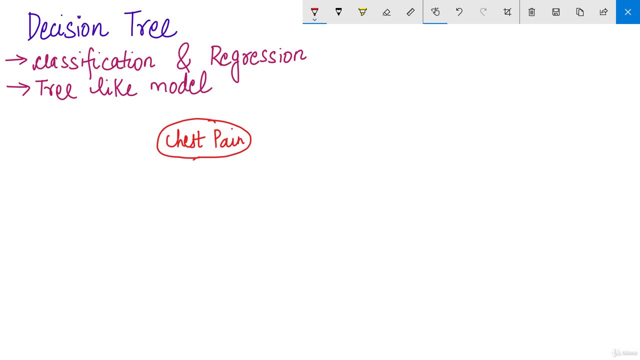 will do is: doctor will first check his BP, right, like most of almost all the doctors check BP first and then the stethoscope. they used to do the heart rate and everything. so if the BP is there, like maybe a high or low, like it is, it comes into this branch. a BP is the BP is coming into high or low, whatever. 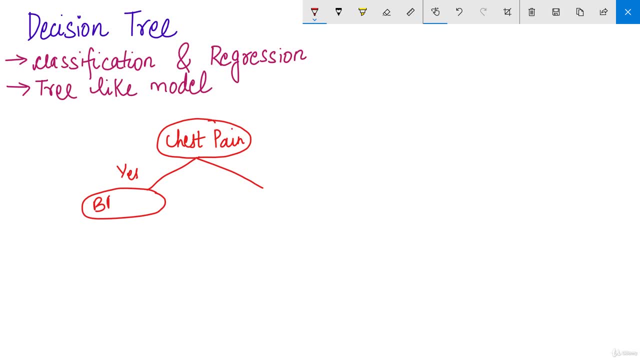 it is it. he will suggest like it will say it is a BP problem and it was, and I just tell you what will happen next. and if it's no, then he'll check, let's say pulse, like. sorry guys, I'm not into medical domain, I have no idea what exactly it is, but I'm just trying to. 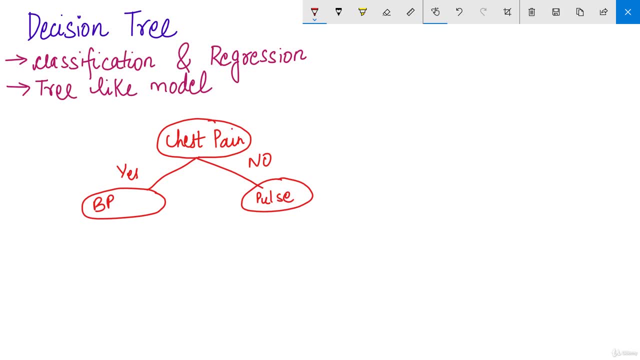 explain you what this entry looks like. so like if you go to a doctor and you says, doctor, I have a chest pain, so he will say, okay, let me check your BP. if there is a BP low or BP yes, then again there will be two like there is a BP. 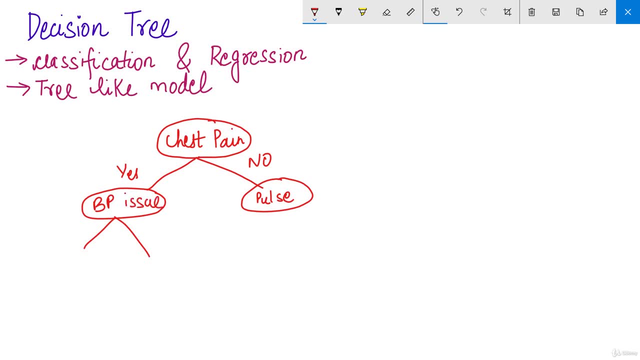 let's say issue. so now BP issue. BP can be low. BP can be high. so now BP issue. BP can be low. BP can be high. so now BP issue. BP can be low. BP can be high. if BP is low, he will suggest let's. if BP is low, he will suggest let's. 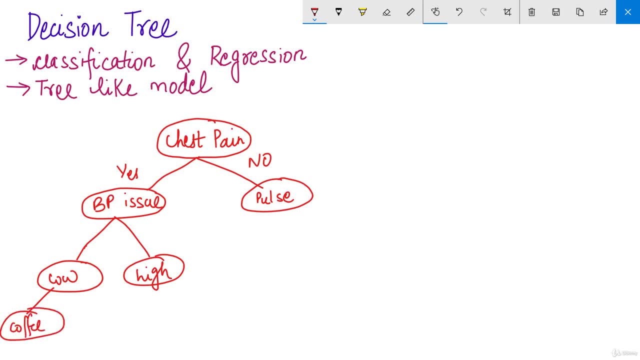 if BP is low, he will suggest, let's say, drink coffee and eat salty foods- right, say, drink coffee and eat salty foods- right, say, drink coffee and eat salty foods- right, whatever I know. and if BP is high, whatever I know, and if BP is high, whatever I know, and if BP is high, he will suggest, like, go for this test. or 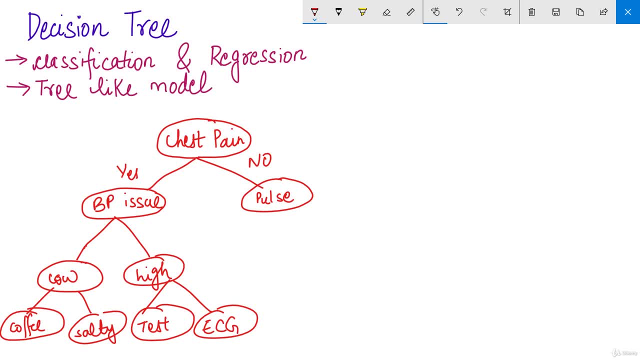 he will suggest like: go for this test. or he will suggest like: go for this test, or let's do a ECG as well for chest pain. let's do a ECG as well for chest pain. let's do a ECG as well for chest pain. and 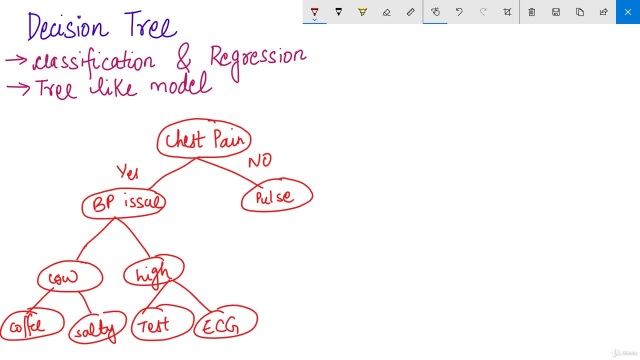 and and and. if there is no BP issue, he'll check the. if there is no BP issue, he'll check the. if there is no BP issue, he'll check the pulse. if the pulse is normal when once pulse. if the pulse is normal when once pulse, if the pulse is normal when once there will be a normal pulse, then he'll. 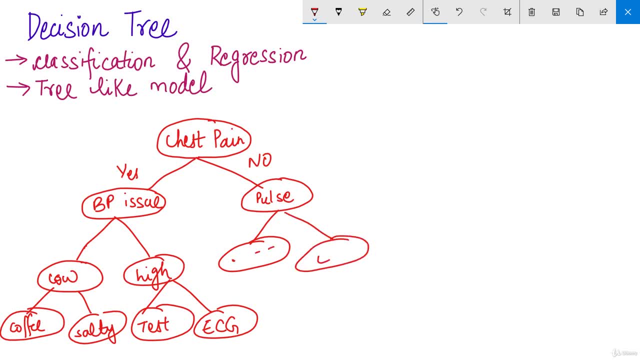 there will be a normal pulse, then he'll. there will be a normal pulse, then he'll suggest some other thing. and if the suggest some other thing, and if the suggest some other thing, and if the pulse is high, he'll again suggest ECG. and pulse is high, he'll again suggest ECG. and 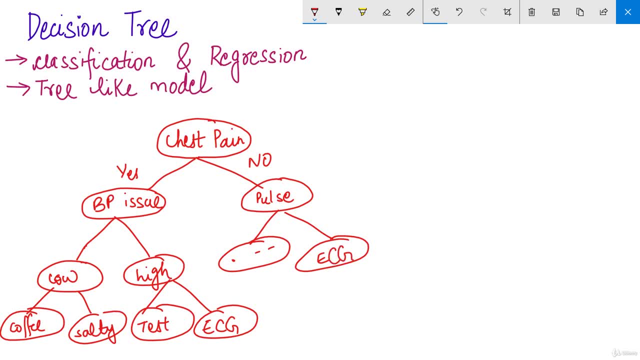 pulse is high. he'll again suggest ECG and similar thing. I hope you understanding similar thing. I hope you understanding similar thing. I hope you understanding. so this is what a decision tree looks. so this is what a decision tree looks. so this is what a decision tree looks like. finally, he will be coming at a 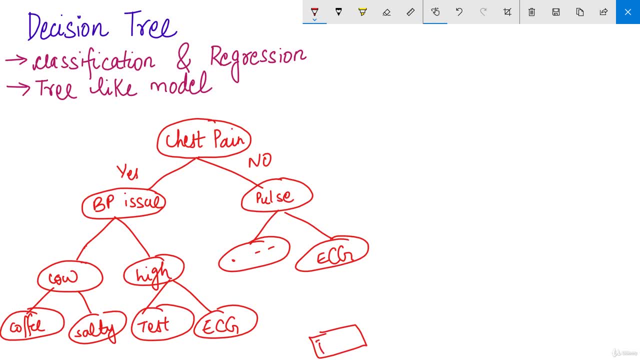 like: finally, he will be coming at a like, finally, he will be coming at a point at last, and he will be telling point at last. and he will be telling point at last, and he will be telling: like there will be a result at the last, like there will be a result at the last. 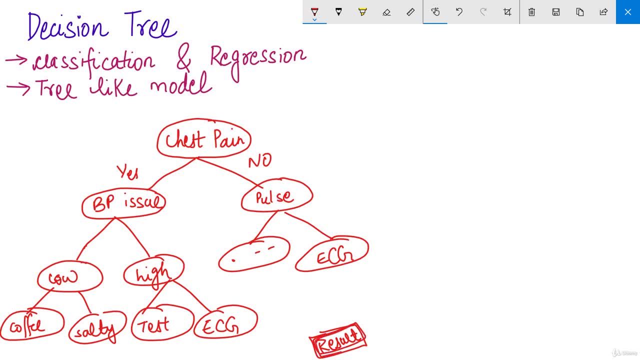 like. there will be a result at the last and he will get to know that what, and he will get to know that what, and he will get to know that what exactly is happening with the patient exactly is happening with the patient, exactly is happening with the patient become, and why there is a chest pain. so 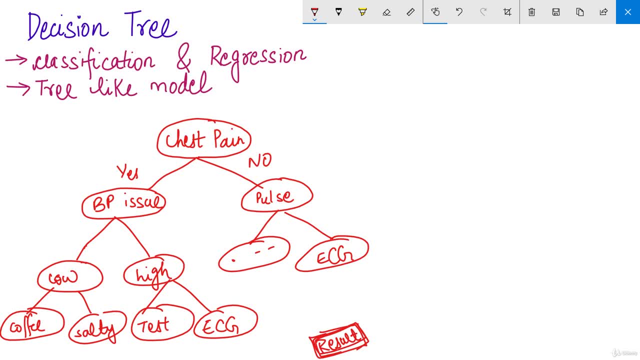 become and why there is a chest pain. so become and why there is a chest pain, so he will get to know at last, right, so he will get to know at last, right, so he will get to know at last, right. so this is how, like basically all on daily. 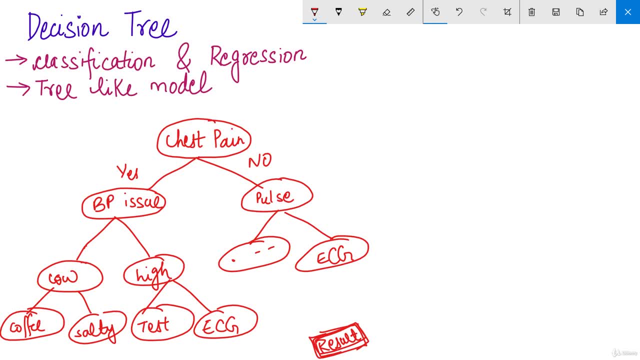 this is how like, basically all on daily. this is how like, basically all on daily basis, like each and every of us. if you basis like each and every of us, if you basis like each and every of us, if you want to take a decision, some, some other, 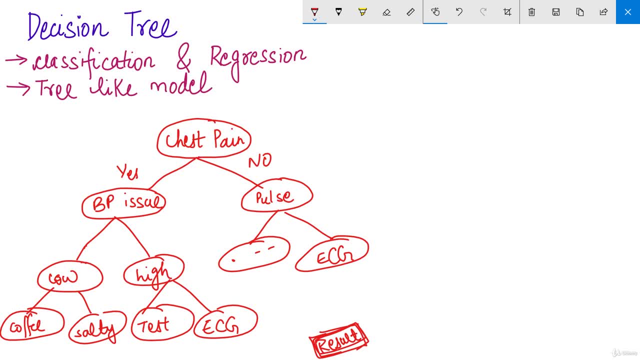 want to take a decision. some, some other want to take a decision, some some other other way. we do somewhat like this, we other way. we do somewhat like this, we other way. we do somewhat like this. we just don't make a tree or a flow chart. just don't make a tree or a flow chart. 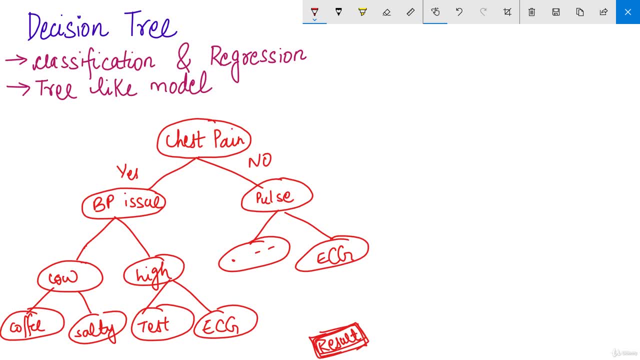 just don't make a tree or a flow chart like this, but we do right, so this was like this, but we do right, so this was like this, but we do right. so this was the best example which I can come up, the best example which I can come up. 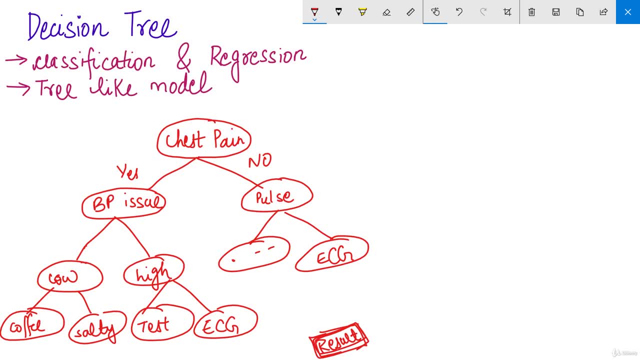 the best example which I can come up with to explain the decision tree. this with: to explain the decision tree. this with: to explain the decision tree: this is how decision tree looks like. so this is how decision tree looks like. so this is how decision tree looks like. so this is just an example. so, and these are like 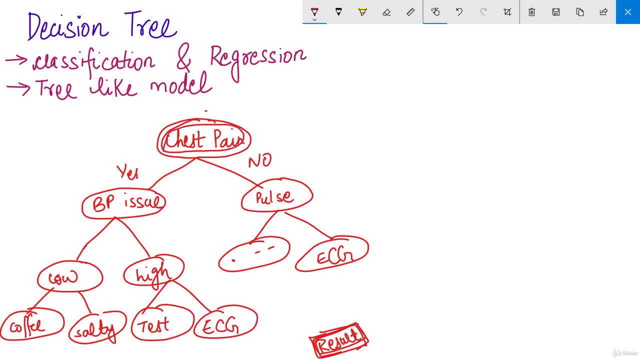 is just an example, so. and these are like is just an example so. and these are like in decision tree. these are like your in decision tree. these are like your in decision tree. these are like your root note, and also one more thing: our root note, and also one more thing: our. 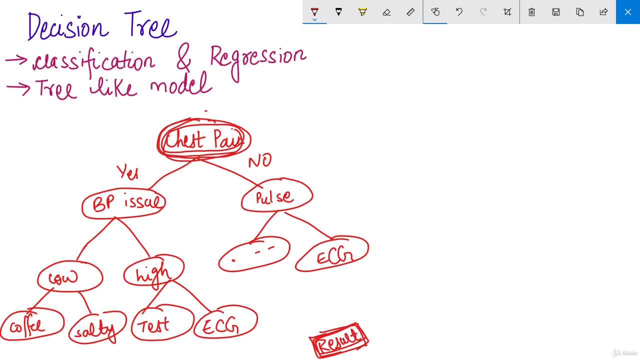 root note. and also one more thing: our tree is upside down, like roots are at. the tree is upside down like roots are at. the tree is upside down like roots are at the top- just make a note of this. roots are top, just make a note of this. roots are. 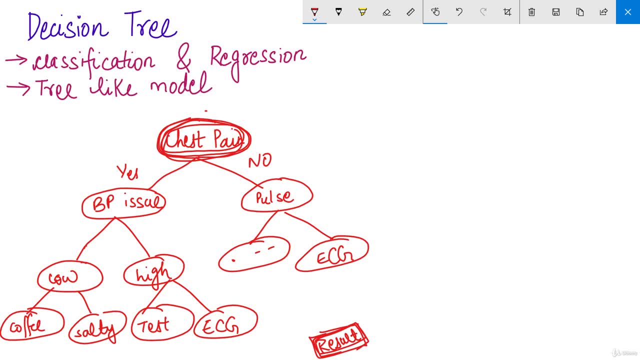 top. just make a note of this. roots are at the top and these are the leaves, so at the top, and these are the leaves, so at the top, and these are the leaves. so it is upside down and this is a like. it is upside down and this is a like. 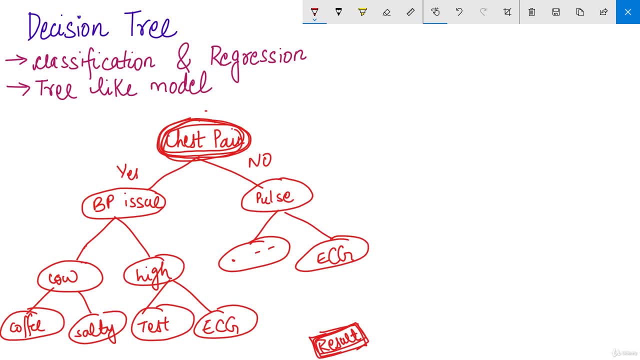 it is upside down, and this is a like root node or a parent node, and these are root node or a parent node, and these are root node or a parent node, and these are the child nodes, that which are carrying the child nodes, that which are carrying the child nodes, that which are carrying forward at the bottom. so, if I want to, 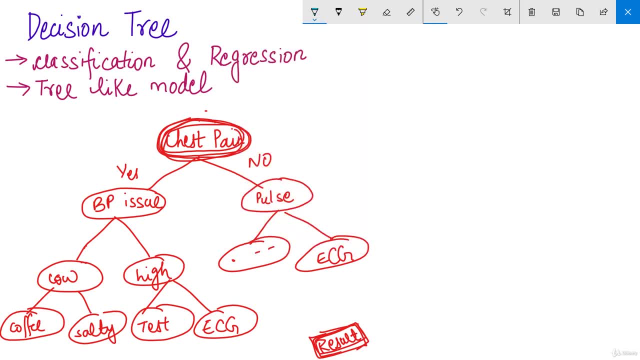 forward at the bottom. so if I want to forward at the bottom, so if I want to explain one more example, a very simple, explain one more example. a very simple, explain one more example, a very simple example. let me tell you: okay, so let's example. let me tell you, okay, so let's. 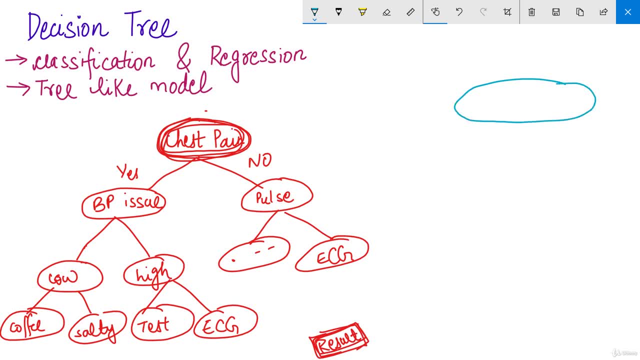 example, let me tell you: okay. so let's say: like our person is going to buy a say, like our person is going to buy a say, like our person is going to buy a flat or a room like not a room, or like flat or a room like not a room, or like. 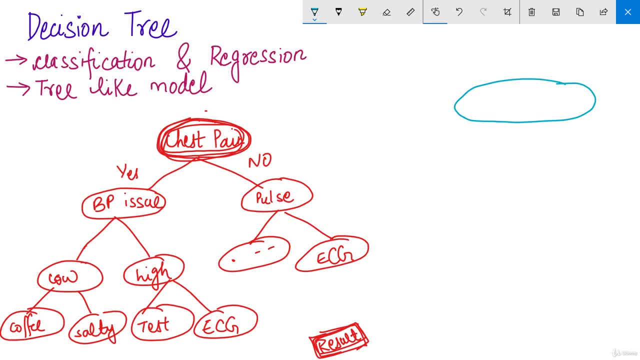 flat or a room like not a room, or like that's a house or a flat somewhere, so that's a house or a flat somewhere, so that's a house or a flat somewhere. so he'll like this, this house, have more. he'll like this, this house, have more. 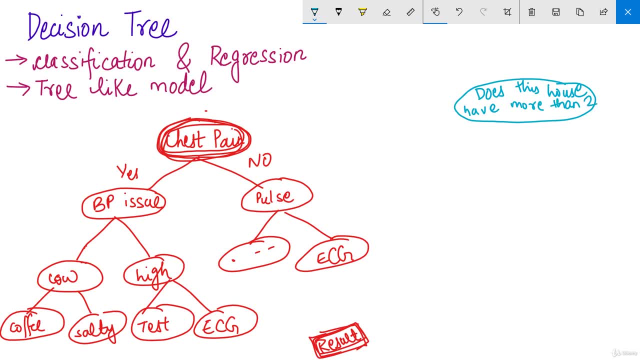 he'll like this: this house have more then two rooms, then two rooms, then two rooms if that flat has more than two rooms. like if that flat has more than two rooms. like if that flat has more than two rooms. like if there is no like. no, there is no more. 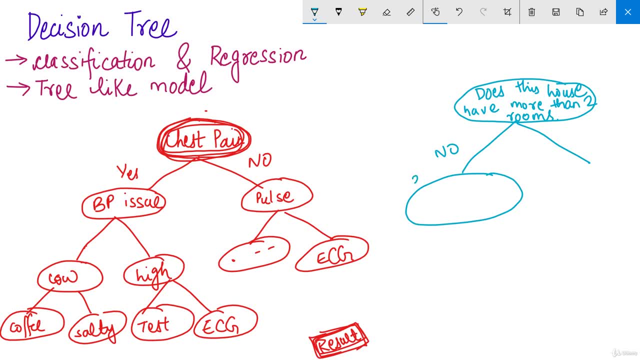 if there is no like no, there is no more. if there is no like no, there is no more than two room. it's a 2bhk flat. no, it's than two room. it's a 2bhk flat. no, it's than two room, it's a 2bhk flat. no, it's a 2bhk flat. so your predicted price is: 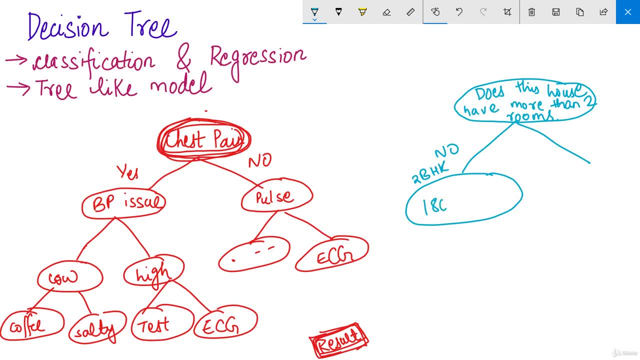 a 2bhk flat. so your predicted price is a 2bhk flat. so your predicted price is: let's say this was dollars and yes, it. let's say this was dollars and yes, it. let's say this was dollars and yes, it has it is a 3bhk. 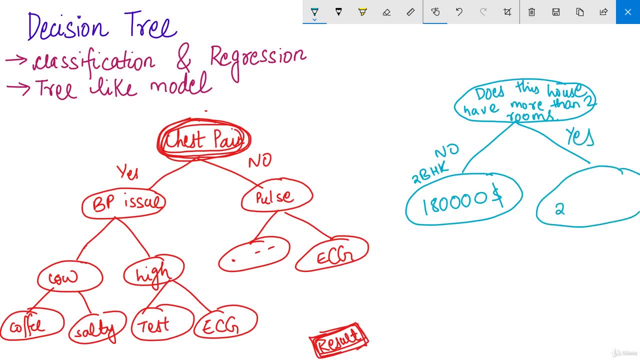 has it is a 3bhk. has it is a 3bhk flat or 4bhk flat, then the predicted price is flat. or 4bhk flat, then the predicted price is flat, or 4bhk flat, then the predicted price is: let's say this much. so this is: 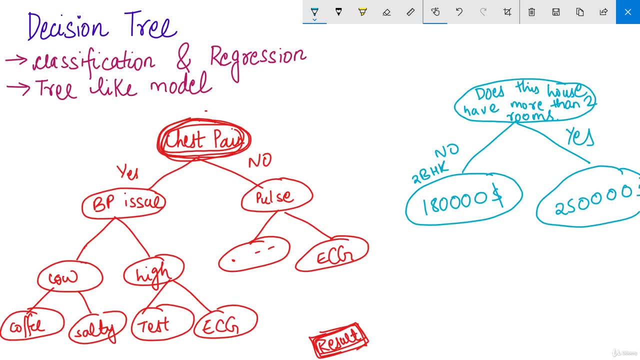 let's say this much, so this is. let's say this much, so this is again: we can simplify it. we can create more again. we can simplify it. we can create more again. we can simplify it. we can create more branches to it. like: okay, if it's 2bhk. 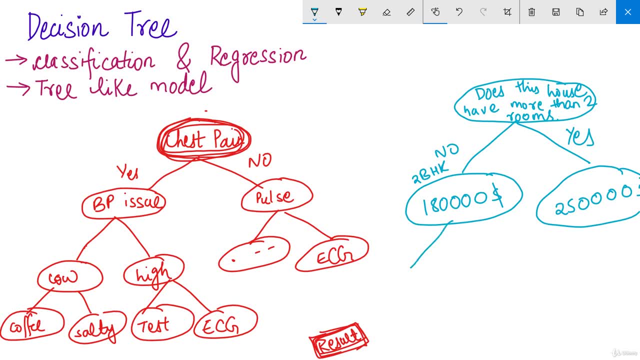 branches. to it like: okay if it's 2bhk branches. to it like: okay if it's 2bhk flat, the washrooms are attached to each flat. the washrooms are attached to each flat. the washrooms are attached to each room or there is a single washroom, like 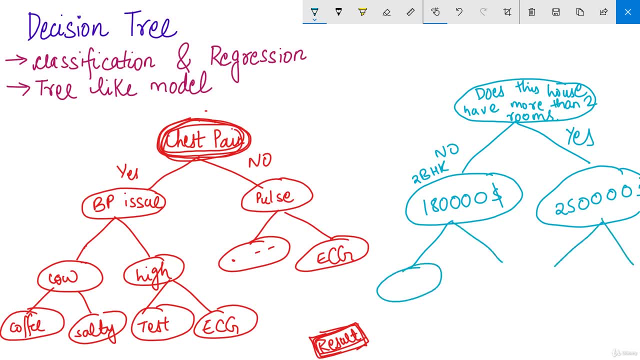 room, or there is a single washroom like room, or there is a single washroom like this: we can subdivide it, and again so this, we can subdivide it, and again so this, we can subdivide it, and again so. this is how decision tree can grow up, and 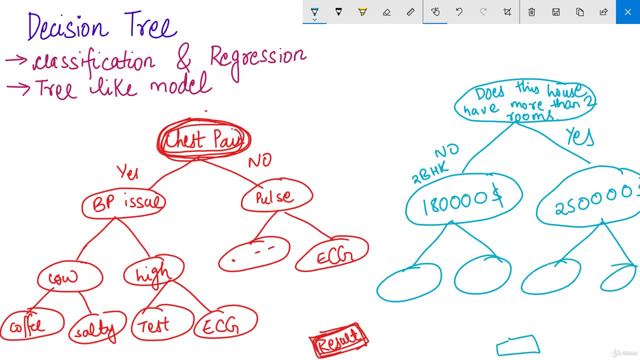 this is how decision tree can grow up, and this is how decision tree can grow up and finally like a person. okay, we can finally like a person. okay, we can finally like a person. okay, we can decide like which one, which one he can, decide like which one, which one he can. 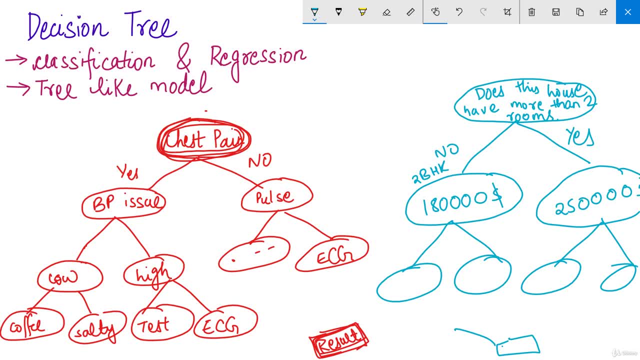 decide like which one, which one he can buy. so this is this. I'm giving an buy. so this is this, I'm giving an buy. so this is this. I'm giving an example how decision tree looks like. example. how decision tree looks like. example. how decision tree looks like. somewhat looks like. I hope are you. 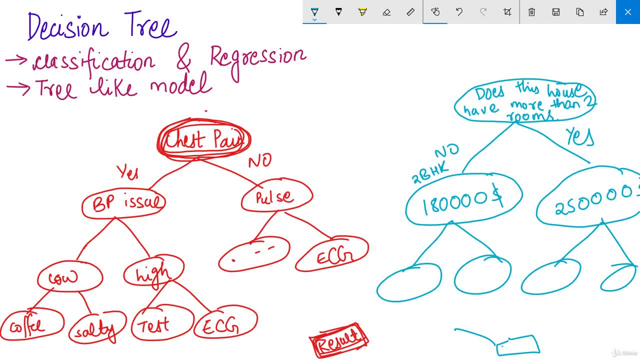 somewhat looks like I hope. are you somewhat looks like I hope? are you clear up to this, okay? so, basically, clear up to this, okay. so, basically clear up to this, okay. so basically, decision tree naturally represents the decision tree naturally represents the decision tree naturally represents the way we make decisions in our day-to-day. 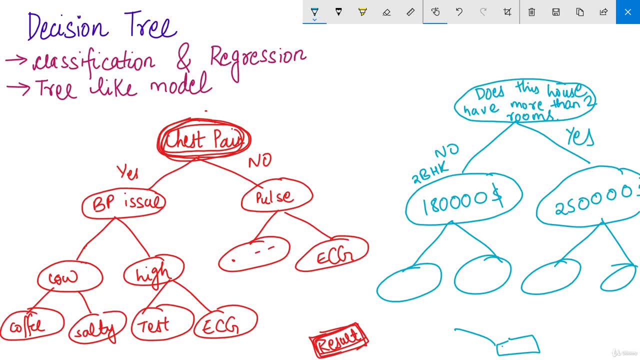 way we make decisions in our day-to-day way, we make decisions in our day-to-day life right. so this is the example which life right. so this is the example which life right. so this is the example which I am showing you here right now is. I am showing you here right now is. 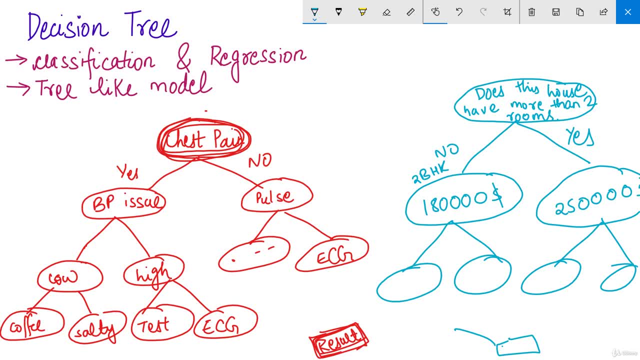 I am showing you here right now is nothing but our decision, which make we nothing but our decision, which make we nothing, but our decision, which make we make in our day-to-day life. so this make in our day-to-day life, so this make in our day-to-day life, so this entry, are easy to understand and they. 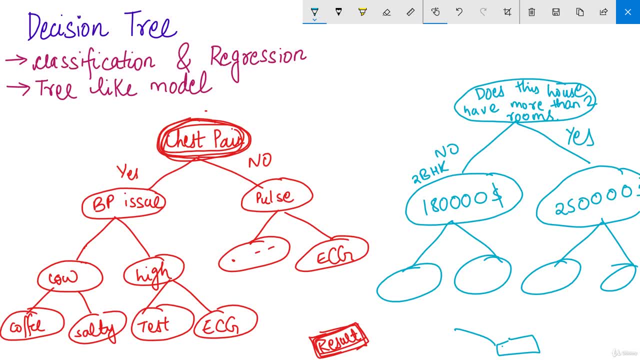 entry are easy to understand and they entry are easy to understand and they are the basic building block for some of are the basic building block for some. of are the basic building block for some of the best models in data science right- the best models in data science right. 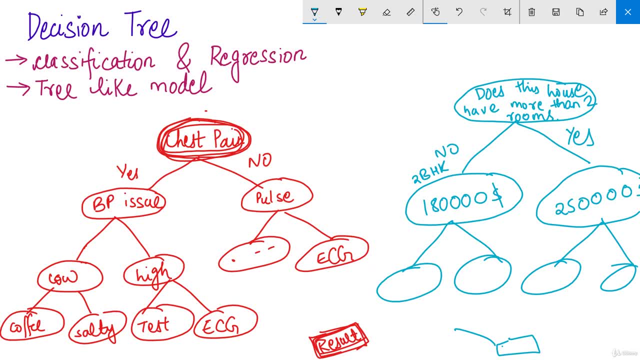 the best models in data science. right, but if you are very thorough with but if you are very thorough with, but if you are very thorough with decision tree it. they are like the decision tree it. they are like the decision tree it. they are like the building blocks of one of the best. 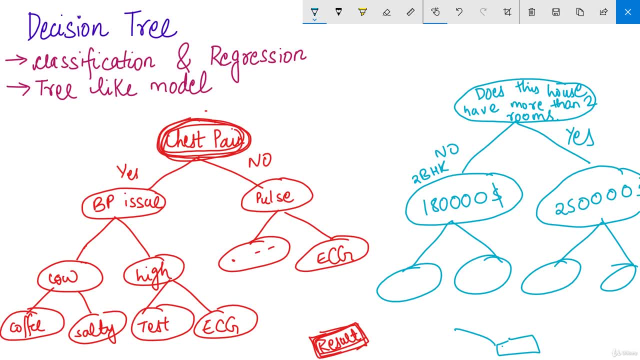 building blocks of one of the best building blocks of one of the best project to work on in data science stream. project to work on in data science stream. project to work on in data science stream. if you are good with decision tree, you. if you are good with decision tree, you. 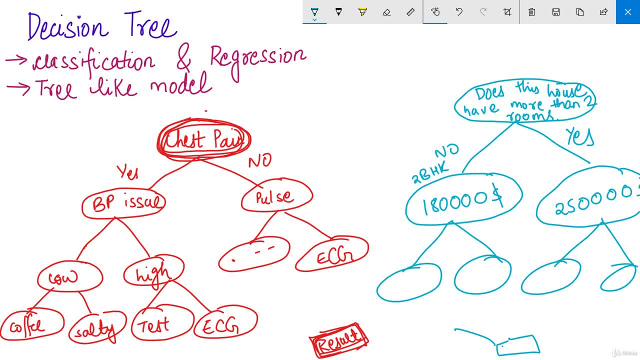 if you are good with decision tree, you can build one best decision tree model. can build one best decision tree model. can build one best decision tree model or something so in decision tree like, or something so in decision tree like, or something so in decision tree like there are. there is one benefit, like if 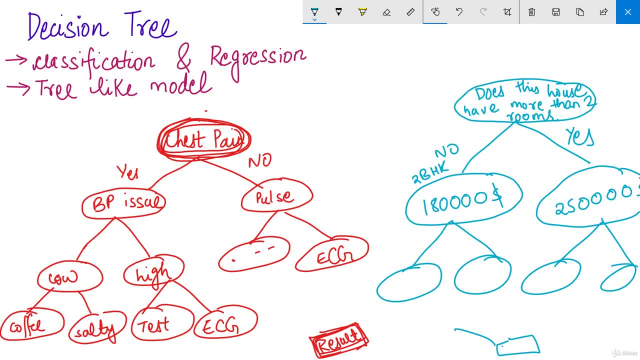 there are. there is one benefit like: if there are. there is one benefit like: if you remember in your logistic regression, you remember in your logistic regression, you remember in your logistic regression like I have explained you in my logistic, like I have explained you in my logistic, like I have explained you in my logistic regression: with lecture you can only get. 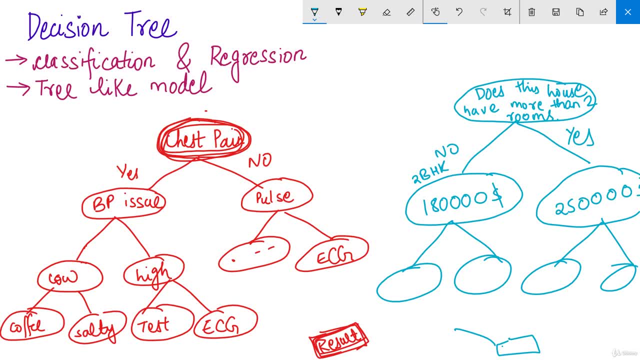 regression with lecture. you can only get regression with lecture. you can only get some sort of linear boundary condition, some sort of linear boundary condition, some sort of linear boundary condition. you, if you, I hope you remember linear. you, if you, I hope you remember linear. you, if you, I hope you remember linear boundary condition. and let me just show: 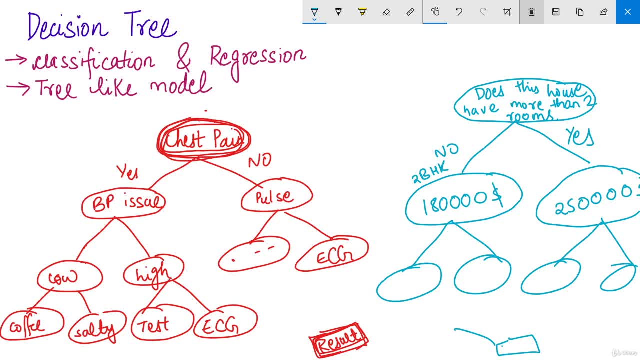 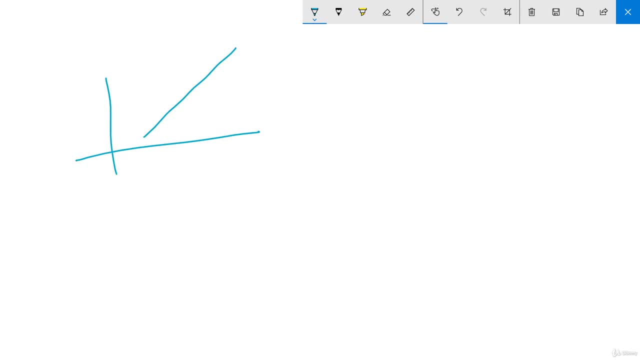 boundary condition, and let me just show boundary condition and let me just show you, let me erase this somewhat like this. you let me erase this somewhat like this. you let me erase this somewhat like this: if you remember, in in our logistic, if you remember in in our logistic, 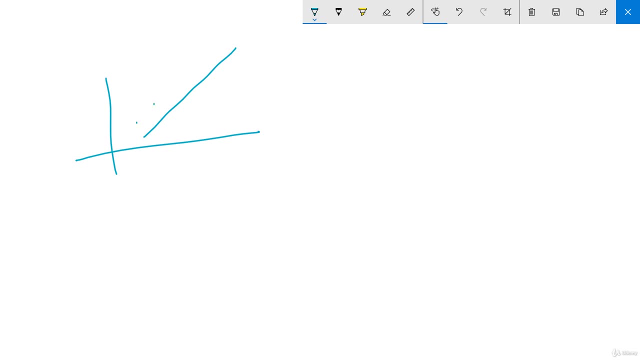 if you remember, in in our logistic regression there was a linear boundary regression. there was a linear boundary regression. there was a linear boundary condition, right, but in decision tree you condition right, but in decision tree you condition right, but in decision tree you can also get nonlinear boundary. 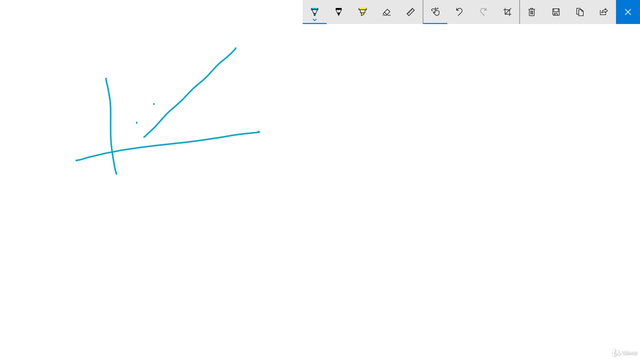 can also get nonlinear boundary, can also get nonlinear boundary conditions. why like you your question conditions? why like you your question conditions? why like you? your question was: why and how? because you can see in was why and how. because you can see in was why and how. because you can see in this entry: we are not own there like we. 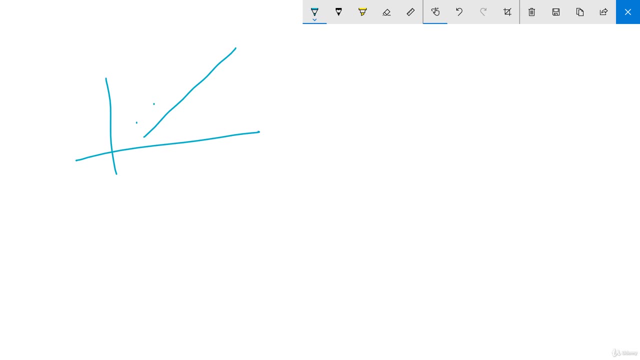 this entry. we are not own there, like we. this entry, we are not own there, like we are not only focusing on into the are not only focusing on into the, are not only focusing on into the probabilities which are occurring in fact, probabilities which are occurring in fact. 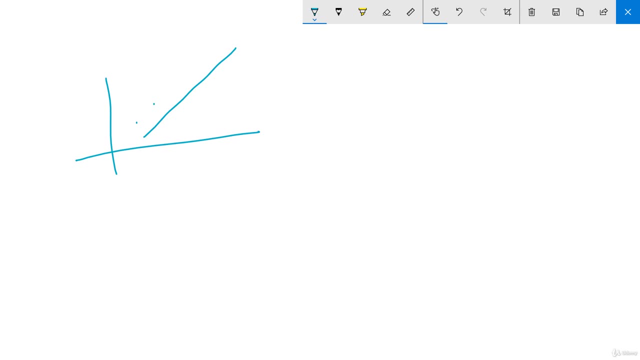 probabilities which are occurring. in fact, we are drawing a tree to get even. we are drawing a tree to get even. we are drawing a tree to get even nonlinear data and also we can get some nonlinear data and also we can get some nonlinear data and also we can get some meaningful information out of that. we. 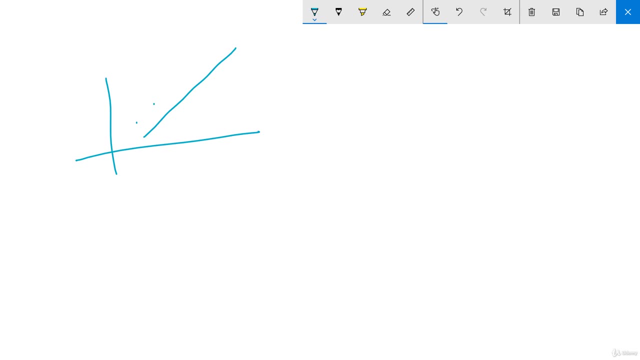 meaningful information out of that we meaningful information out of that we are not completely based on, are not completely based on, are not completely based on probabilities here, like we are creating probabilities here, like we are creating probabilities here, like we are creating trees, branches, and there are many other. 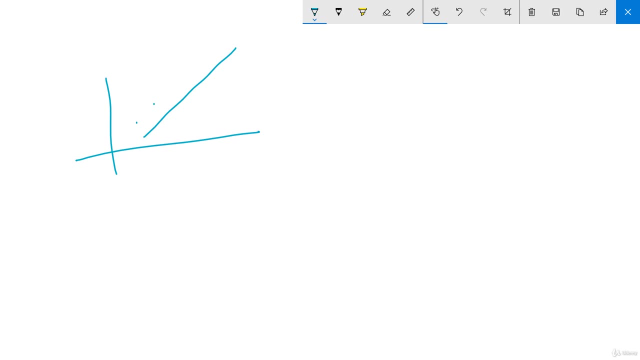 trees, branches, and there are many other trees, branches and there are many other things that you will understand in things that you will understand in things that you will understand in coming like in future. so what next also coming like in future? so what next also coming like in future? so what next also, like I can tell you, like in decision. 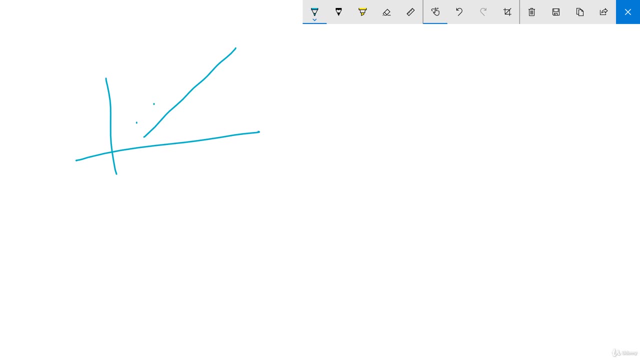 like I can tell you like in decision, like I can tell you like in decision, tree can be upgraded, tree can be upgraded, tree can be upgraded like: if this is a decision tree, you like, if this is a decision tree, you like, if this is a decision tree, you understanding decision tree, you can say: 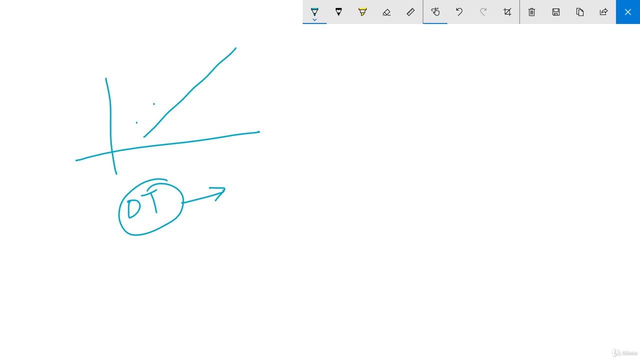 understanding decision tree. you can say: understanding decision tree. you can say it is a. there is a upgradation part of it is a. there is a upgradation part of it is a. there is a upgradation part of decision tree which is known as random decision tree which is known as random. 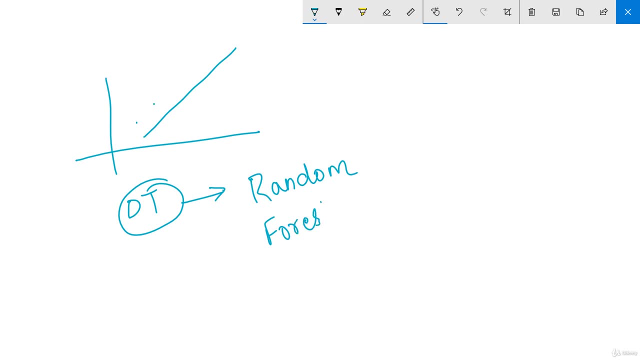 decision tree, which is known as random forest. you can say: if this is your forest. you can say: if this is your forest, you can say: if this is your bachelors, this is your masters of the bachelors, this is your masters of the bachelors, this is your masters of the same thing. and if you are good with 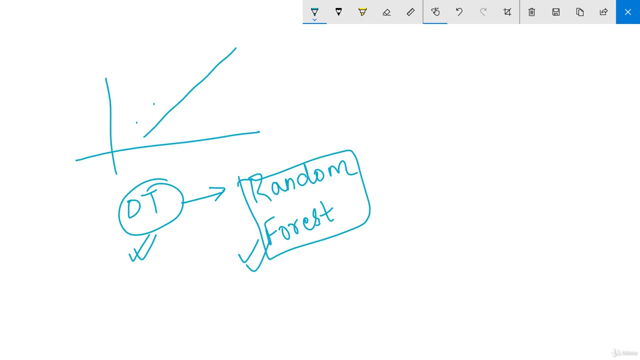 same thing and if you are good with same thing, and if you are good with decision tree, you can easily upgrade decision tree. you can easily upgrade decision tree. you can easily upgrade which is these days very popular, which is these days very popular, which is these days very popular, especially with your, if you are doing, 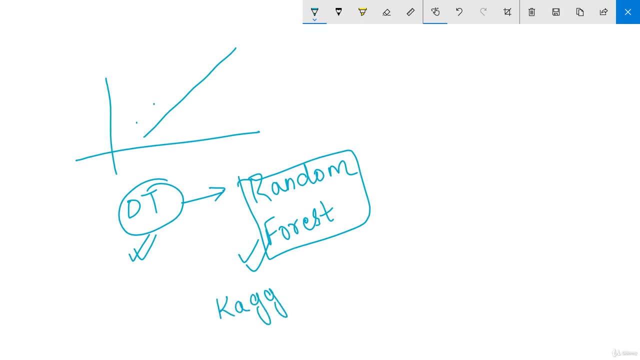 especially with your, if you are doing especially with your, if you are doing projects on your Kaggle Kaggle projects, on your Kaggle Kaggle projects, on your Kaggle Kaggle environment and all like if anyone have environment and all like if anyone have environment and all like if anyone have no idea about Kaggle Kaggle is nothing. 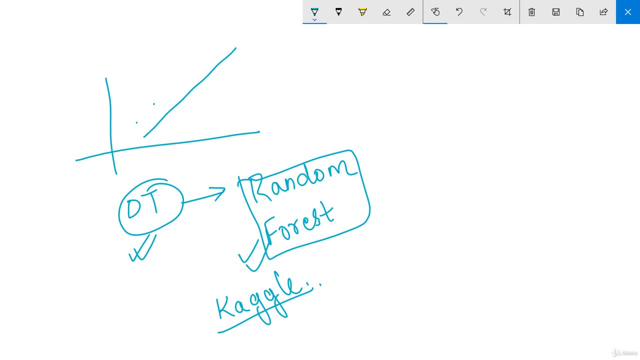 no idea about Kaggle. Kaggle is nothing. no idea about Kaggle. Kaggle is nothing, but our website Kaggle comm where it is. but our website Kaggle comm where it is, but our website Kaggle comm, where it is completely based on data science, where 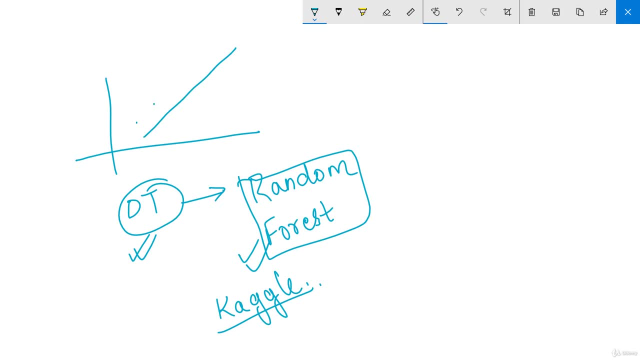 completely based on data science. where, completely based on data science, where you can like, you get a lot of data sets. you can like you get a lot of data sets. you can like, you get a lot of data sets, data frame projects to work on to data frame projects to work on to. 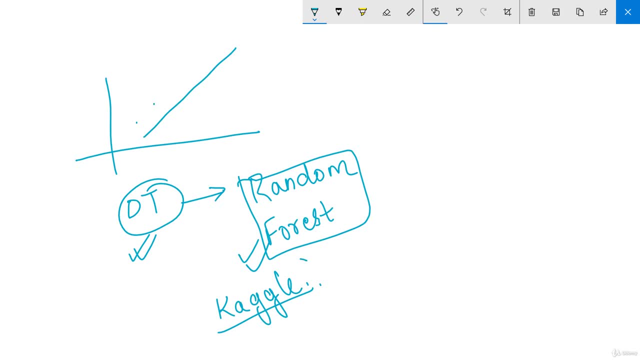 data frame projects to work on, to practice on even companies. they hire on practice on even companies. they hire on practice on even companies. they hire on the basis of Kaggle like whatever. like the basis of Kaggle, like whatever. like the basis of Kaggle like whatever. like they'll say if any company or any client 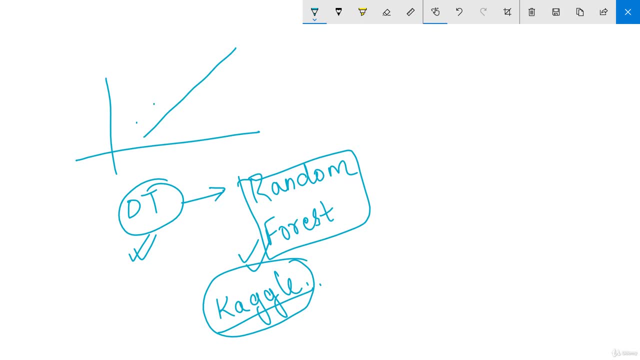 they'll say: if any company or any client, they'll say: if any company or any client have any issue coming up with the have any issue coming up with the have any issue coming up with the project and they are stuck somewhere. project and they are stuck somewhere. 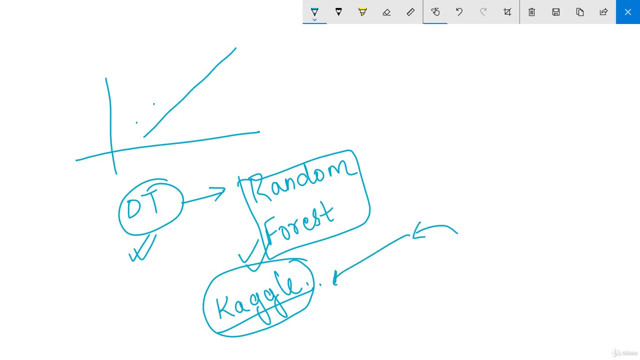 project and they are stuck somewhere, they'll just publish the project into the. they'll just publish the project into the. they'll just publish the project into the into Kaggle, and they'll rate a price like into Kaggle. and they'll rate a price like into Kaggle, and they'll rate a price like, let's say, 10,000 or let's say $1,000. 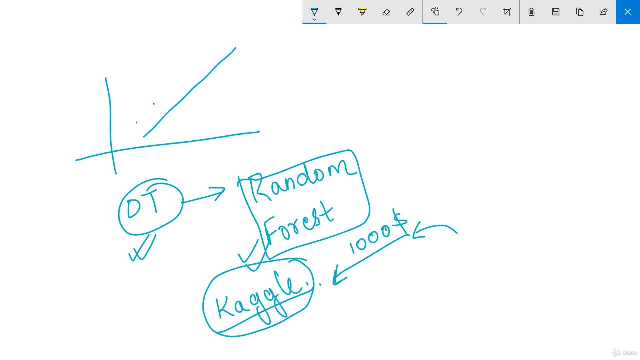 let's say 10,000 or let's say $1,000, let's say 10,000 or let's say $1,000. anyone who solve this problem for me? so anyone who solve this problem for me, so anyone who solve this problem for me, so if like, if you solve the problem ASAP. 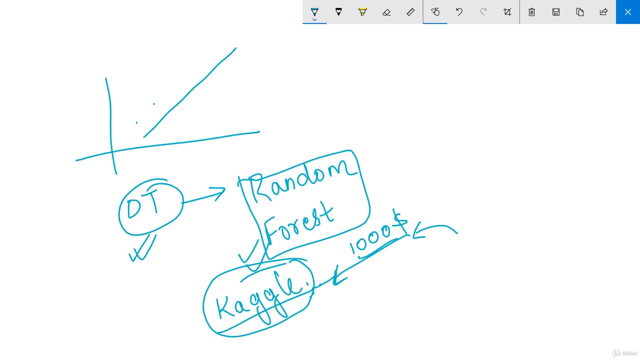 if like, if you solve the problem ASAP, if like, if you solve the problem ASAP and submit back to the person you will and submit back to the person you will and submit back to the person, you will get 10,000, $1,000 like. price varies like. 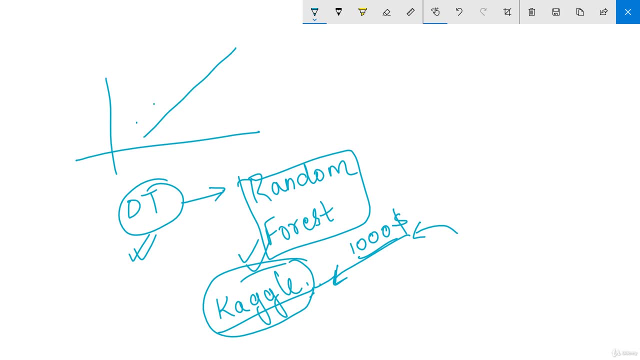 get 10,000 $1,000, like price varies. like get 10,000 $1,000, like price varies. like even I have seen 25,000 price. even you, even I have seen 25,000 price, even you. even I have seen 25,000 price, even you can work in a team and solve the problem. 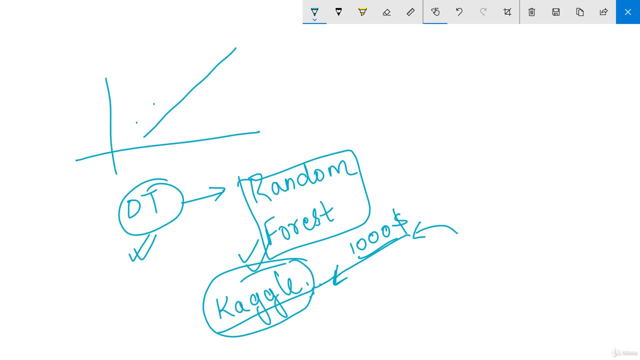 can work in a team and solve the problem, can work in a team and solve the problem, and you can submit that and they'll see. and you can submit that and they'll see. and you can submit that and they'll see. everything is okay and very optimizely. 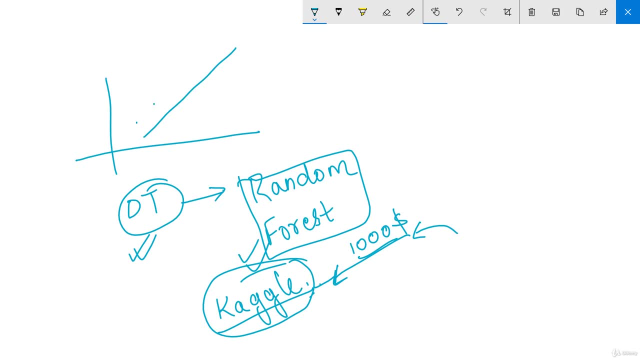 everything is okay and very optimizely. everything is okay and very optimizely. you have like: solved everything, they'll. you have like: solved everything, they'll. you have like: solved everything. they'll. accept your salt project and they'll accept your salt project and they'll. 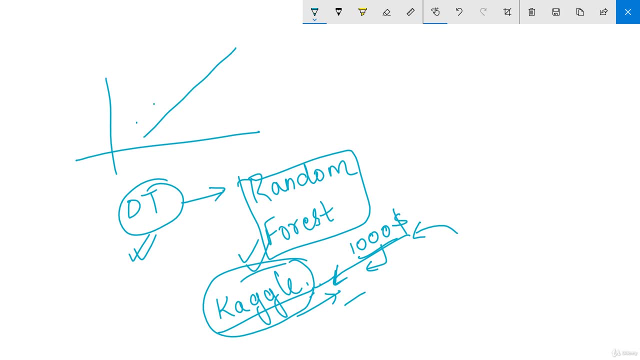 accept your salt project and they'll provide you the money, even if they like. provide you the money, even if they like. provide you the money. even if they like you, they can hire you. if you want you, you, they can hire you. if you want you, you, they can hire you. if you want, you can get hired with them or not, you can. 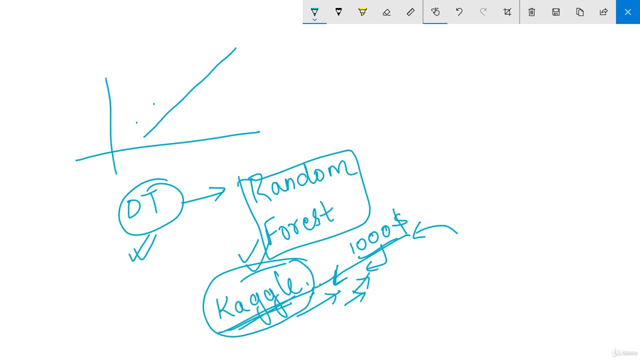 can get hired with them or not. you can can get hired with them or not, you can. let. you can be a freelancer there kegel. let you can be a freelancer there, kegel. let you can be a freelancer there- kegel. so basically, like, kegel is nothing but a. 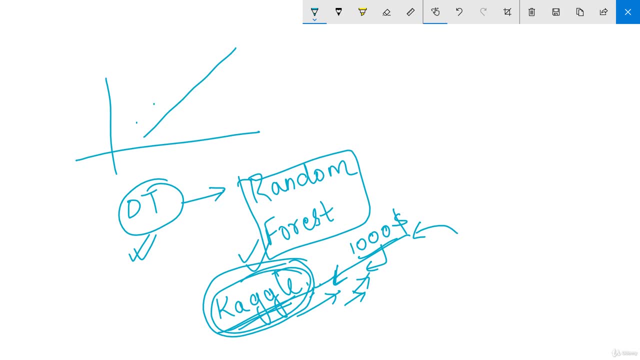 so, basically, like kegel is nothing but a. so, basically, like kegel is nothing but a platform where you work on data science platform, where you work on data science platform, where you work on data science projects and their random forest will be projects and their random forest will be. 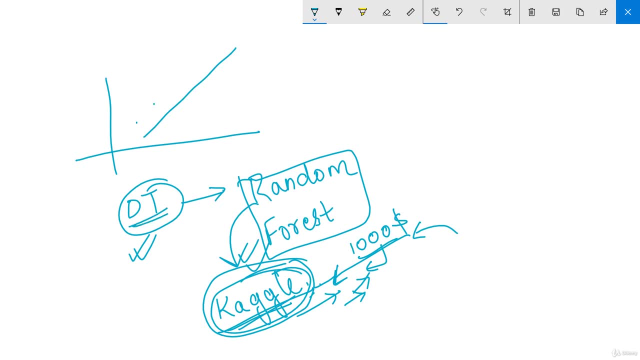 projects and their random forest will be very helpful for you and the basics of very helpful for you and the basics of very helpful for you and the basics of render for us will be coming from your render for us will be coming from your render for us will be coming from your decision to it is and like, if I want to. 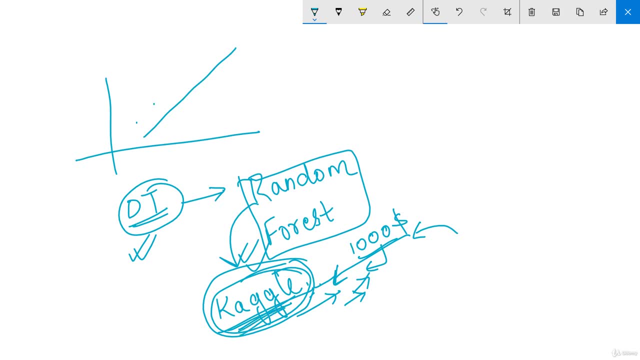 decision to it is, and like: if I want to decision to it is, and like: if I want to say kegel in short, kegel is nothing, but say kegel in short, kegel is nothing but say kegel in short, kegel is nothing. but your compil like it's a competition. 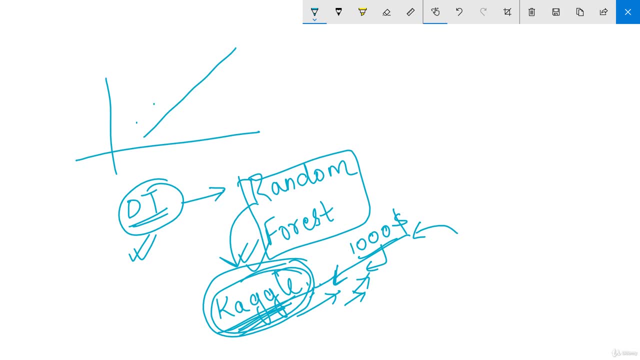 your compil like it's a competition. your compil like it's a competition. forum for data scientists: okay, also one forum for data scientists. okay, also one forum for data scientists. okay, also one more thing like if this is a tree, and more thing like if this is a tree, and 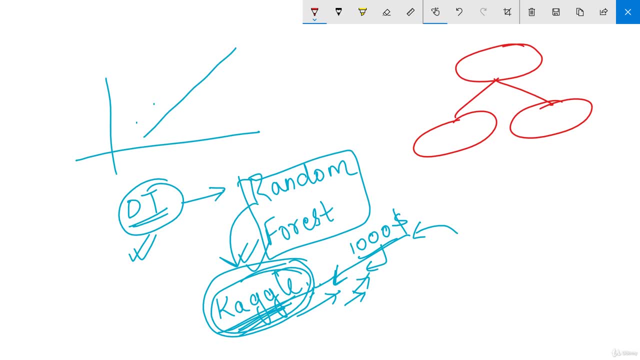 more thing, like if this is a tree, and I've shown you already, shown you, I've shown you already, shown you, I've shown you already shown you examples, and this is our trees, so the examples, and this is our trees, so the examples, and this is our trees, so the data which we provide here at the root. 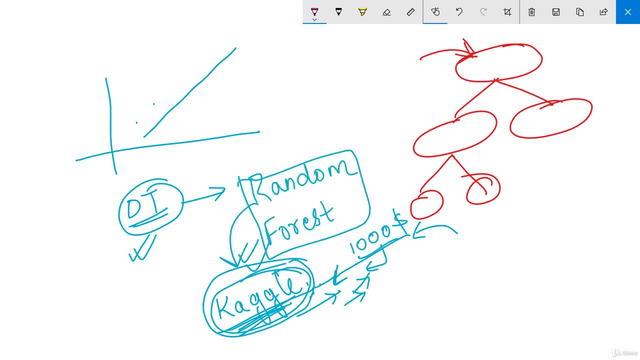 data which we provide here at the root data which we provide here at the root node or the parent node, the data which node or the parent node, the data which node or the parent node. the data which we provide here is the test data now I we provide. here is the test data, now I. 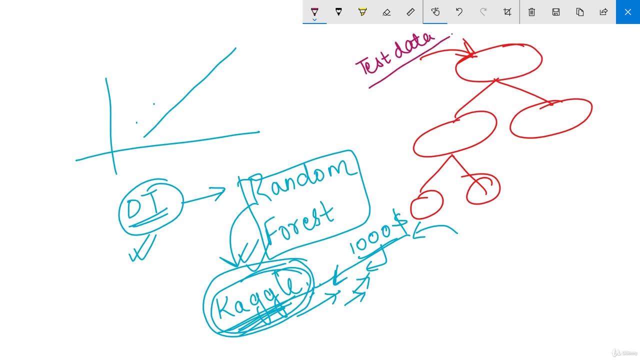 we provide. here is the test data. now, I think everything must be somewhat, the think everything must be somewhat, the think everything must be somewhat. the pictures are somewhat clear into your pictures, are somewhat clear into your pictures, are somewhat clear into your minds, like if it's a test data we are 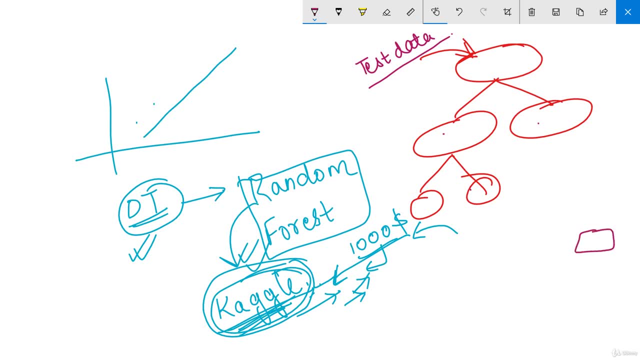 minds like if it's a test data. we are minds like if it's a test data. we are testing some of the other things and testing some of the other things and testing some of the other things and finally coming out with a result at the, finally coming out with a result at the. 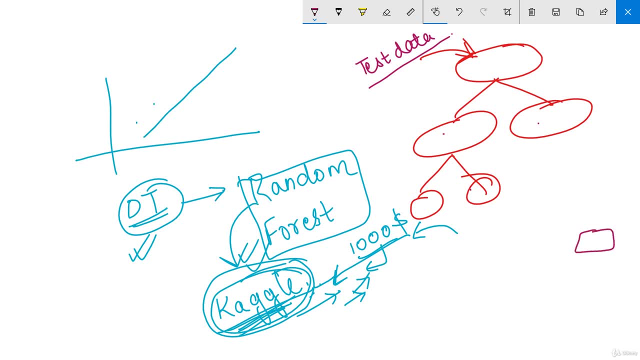 finally coming out with a result at the last. so this is a test data, right guys? last. so this is a test data, right guys? last. so this is a test data, right guys? please make a note. this is a very. please make a note, this is a very. 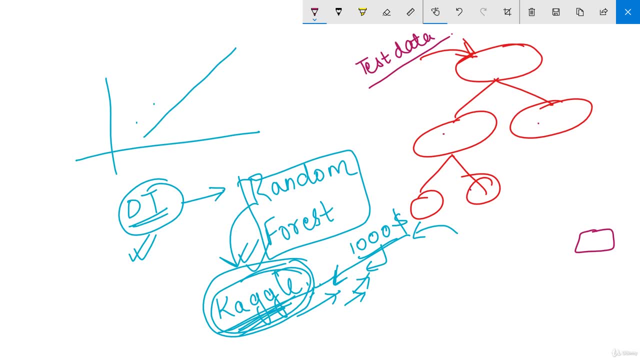 please make a note. this is a very important part of data science, so I want important part of data science. so I want important part of data science, so I want you to make notes of all these. you can you to make notes of all these. you can you to make notes of all these. you can pause the video and make note and then. 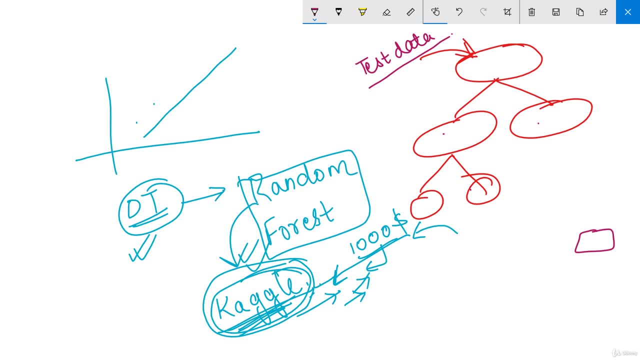 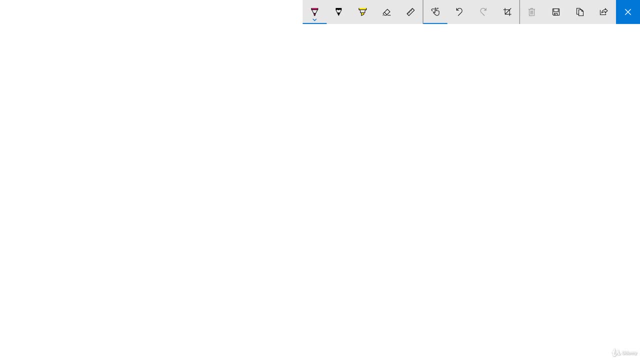 pause the video and make note, and then pause the video and make note, and then you can move forward. okay, so I'll just you can move forward. okay, so I'll just you can move forward. okay, so I'll just erase this. okay, so, decision tree: I'll. 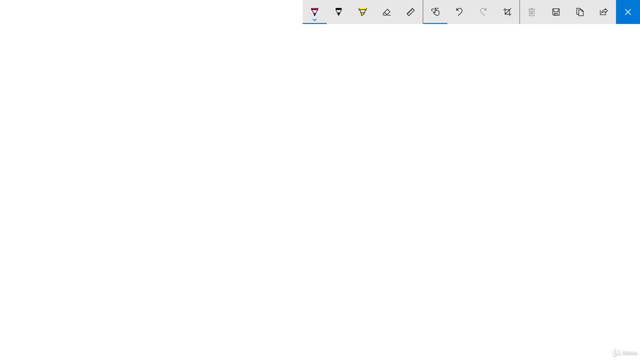 erase this. okay, so decision tree. I'll erase this. okay, so decision tree. I'll denote in short as DT- DT decision trees. denote in short as DT. DT decision trees. denote in short as DT. DT decision trees are also like smooth with categorical. are also like smooth with categorical. 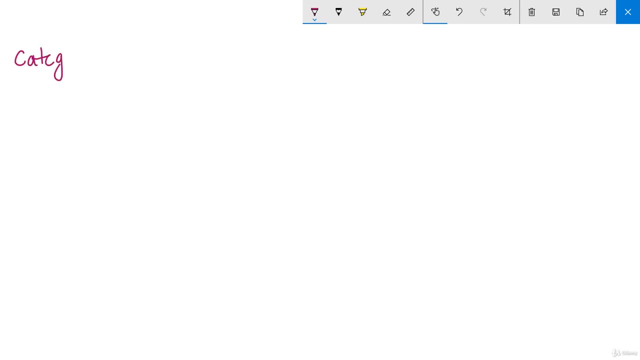 are also like smooth with categorical values. if you remember category values. if you remember category values, if you remember category categorical values in your logistic categorical values, in your logistic categorical values, in your logistic regression there, what what we were doing. regression there, what what we were doing. regression there, what what we were doing in logic logistic regression- if there. 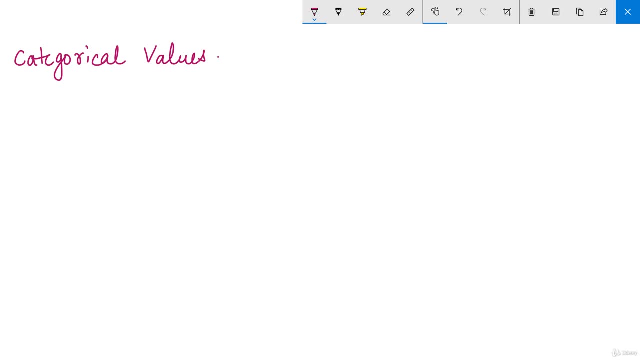 in logic logistic regression. if there in logic logistic regression, if there are categorical values we have to do, are categorical values. we have to do are categorical values. we have to do some of the other thing like dummy part, some of the other thing like dummy part, some of the other thing like dummy part, like one hot encoder or response, and 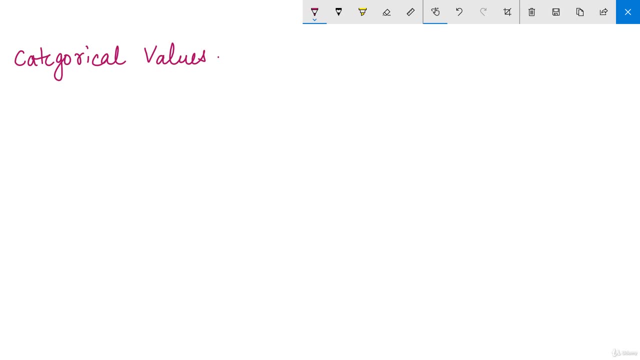 like one hot encoder or response, and like one hot encoder or response and coding. let me just write it down in coding. let me just write it down in coding. let me just write it down in logistic in your logistic regression, if there are, in your logistic regression, if there are. 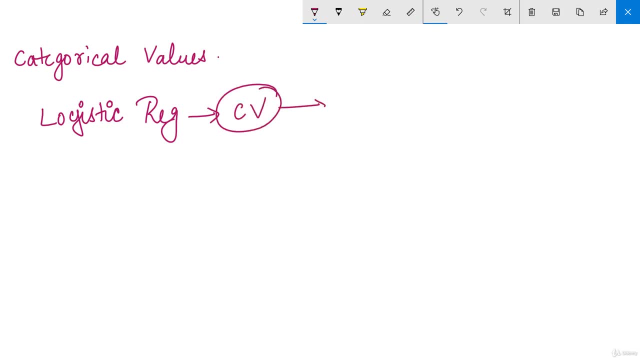 in your logistic regression. if there are categorical values, what we do? we apply categorical values. what we do, we apply categorical values, what we do, we apply one hot. you must have seen in the one hot. you must have seen in the one hot, you must have seen in the project which I have solved. we must have 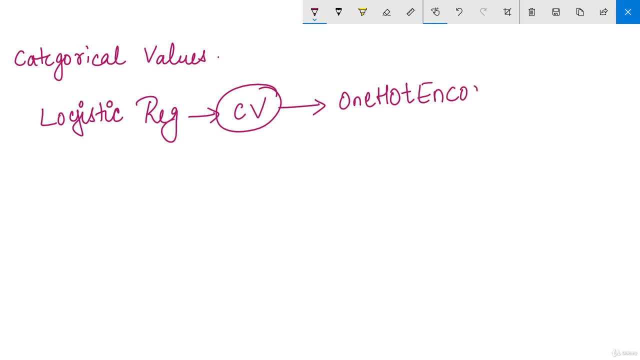 project which I have solved, we must have. project which I have solved, we must have, we must use one hot encoder, or there is, we must use one hot encoder, or there is, we must use one hot encoder, or there is a response, a response, a response encoding, like to solve it, like we logistic. 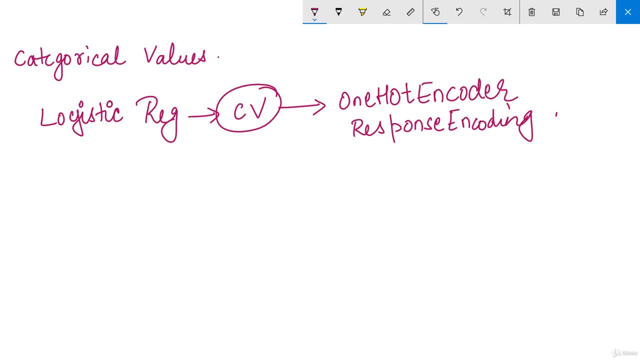 encoding like to solve it like we logistic encoding, like to solve it like we logistic regression. we cannot directly solve the regression. we cannot directly solve the regression. we cannot directly solve the categorical values and using one hot categorical values and using one hot categorical values and using one hot encoder and response encoding, it makes 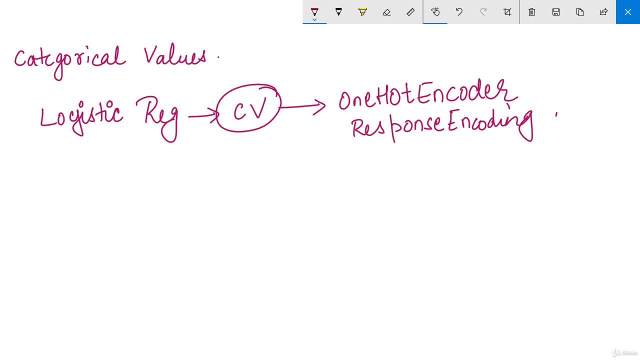 encoder and response encoding. it makes encoder and response encoding. it makes everything like it increases the efforts. everything like it increases the efforts, everything like it increases the efforts. so wherever there is more human effort, so wherever there is more human effort, so wherever there is more human effort, there are more chances of getting errors. 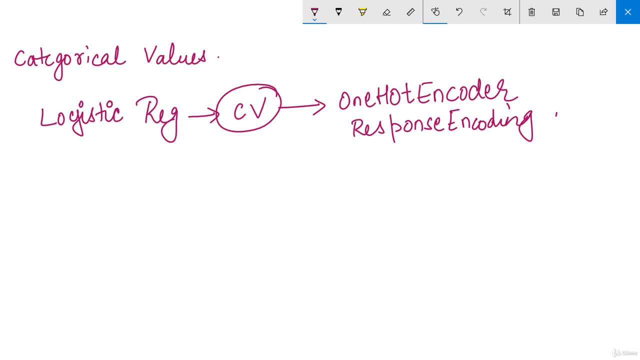 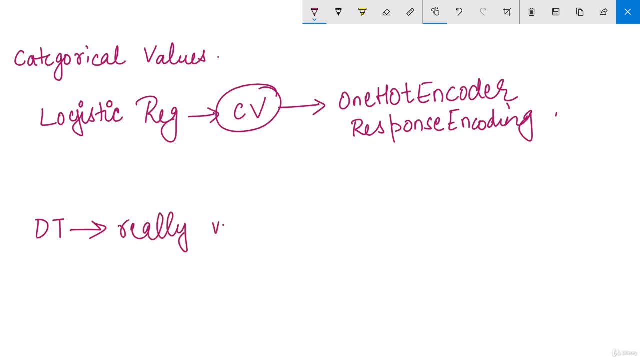 works really really well with categorical values, very well with categorical values, very well with categorical values, very well with categorical values. so this is the one, one of the most. so this is the one, one of the most. so this is the one, one of the most important part of decision tree, like we, 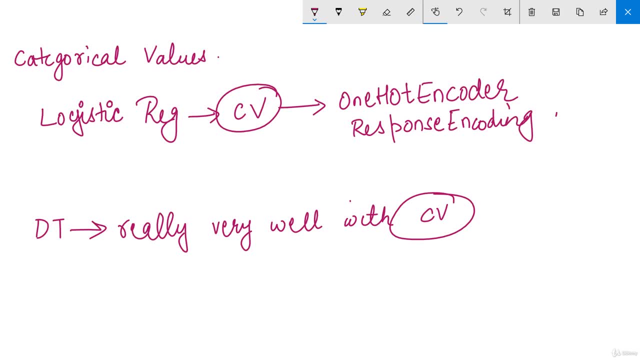 important part of decision tree, like we important part of decision tree. like we don't have to use one hot encoder or don't have to use one hot encoder, or don't have to use one hot encoder or response encoding nothing like that, response encoding nothing like that. 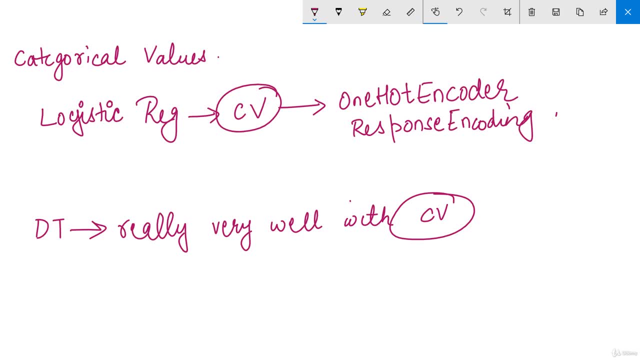 response encoding nothing like that. we just have to assign the value, and we just have to assign the value, and we just have to assign the value, and everything will be covered up. everything will be covered up. everything will be covered up. and also one more thing, and also one more thing. 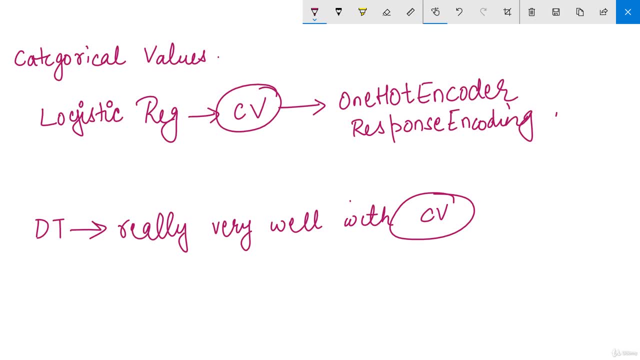 in decision tree usually there is a binary tree like like if this is my root node, and like this is two binary, binary is two, right, so there is a binary tree, but there are chances you can, where you can even expect more than two, like even you can expect three or four, and then if this is if this is the case, it's no. 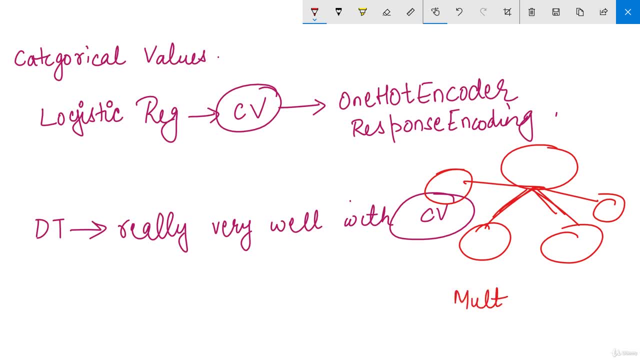 longer binary, it is your multi way splitting. so we say multi way split. so if there are two, this is your binary split, or we call it as binary tree, and if they are more than two, we call it as multi way split. now let me just erase it. 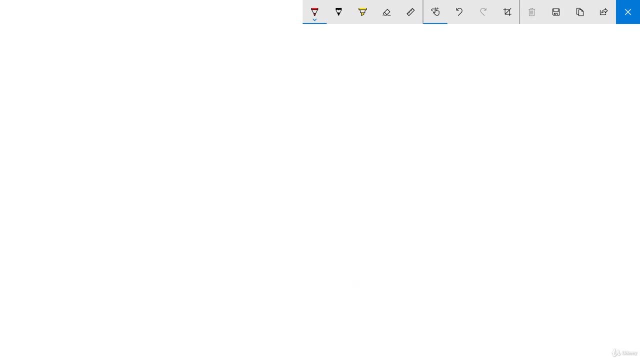 okay. so let me just show you an example from a real data set from one of the medical domain, because in medical domain, usually doctors- like i've shown you an example- he with, he like keep on iterating us, like he keep on asking us, okay, so this has happened to you. so what you ate yesterday, 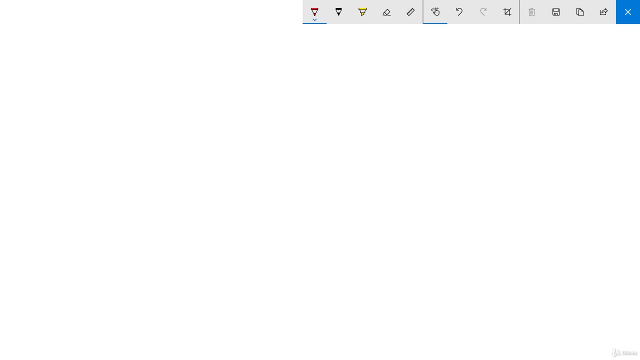 and is there is a fever. so, whatever the reply we give- yes or no basis on the basis of that in his mind he keeps on increasing the branches of the decision tree and finally he comes with a value right? i hope you're getting it what i'm trying to say. so again, i want to give you an 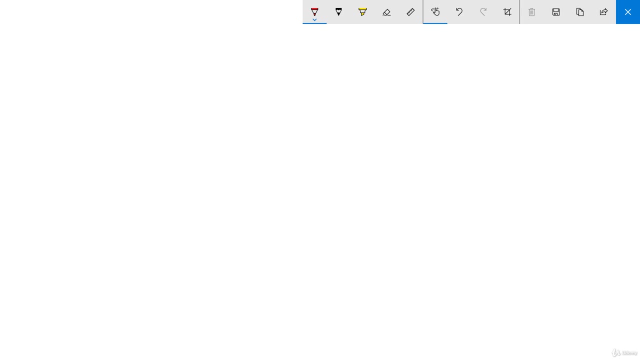 example of a decision tree which is on based on a real data set of medical domain. guys, if you don't know the value, like the terms, medical term, that it's completely okay, you don't have to know the medical terms. but the thing is how decision tree works. i'm going to show. 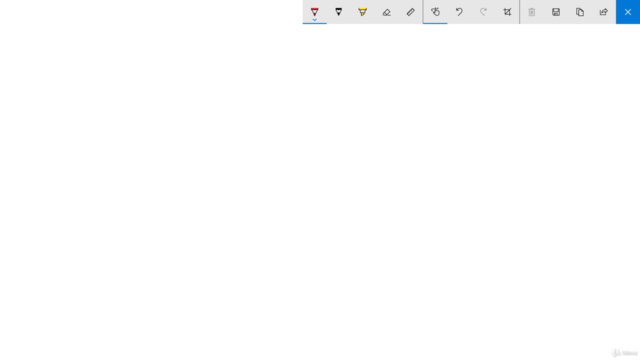 you that. so, in this data set which i'll be, which i have and from which i will be showing you a decision tree, we want to predict whether the patient has a heart disease or not. same thing which i have explained you, but it will be having, it will be a little genuine decision tree having. 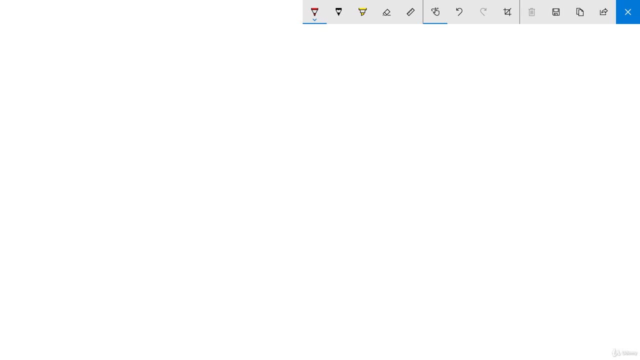 medical words or terminologies, so you can just ignore the medical terms here, all right, so i'll just make a decision tree here. this is something known as thal equals to three. paint type equals to one or two or three, and this is something fluoroscopy. 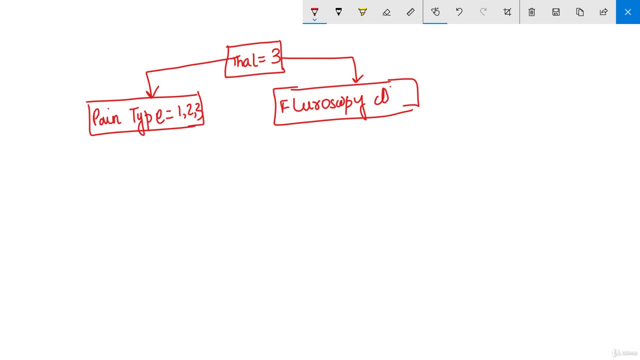 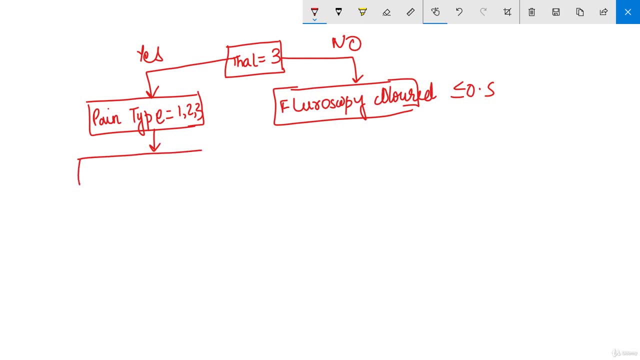 i'll explain you. you can like. it will take like two, three minutes. you can just forward the video where i have completely drawn it, so that you can save time there. itええ, because i can't still remember thal. so to you, pleasechoose a bit more. 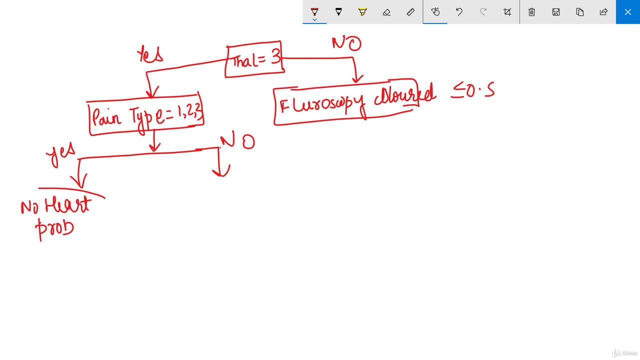 and if it is vér reminder, then all of the things that you can do. i'll explain them all as an example. Ziel avenged problem? yes, no, so there is no heart problem if pain type is not among one, two, three. so again, you have to go for fluoroscopy covered which is less than 0.5 to co kunt. 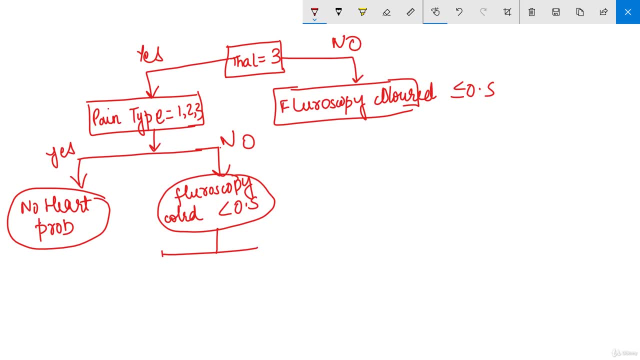 and if it comes to be yes, so there is no heart issue. if it comes as no, there is a heart issue. I don't know how what's happening here, but it's a good example to extend decision tree. no, yes, so there is a heart disease here. enigma exercise. 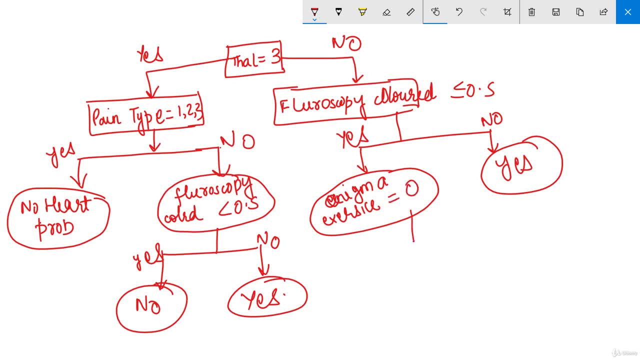 as a zero. yes, no, yes, if age is greater than or equals to 51, why 51? they can even take 50. okay, yes, taken 51. so again, there is a subdivision. if, yes, yes, there is no heart disease, no, there is a heart disease. so, guys, this is a complicated decision. 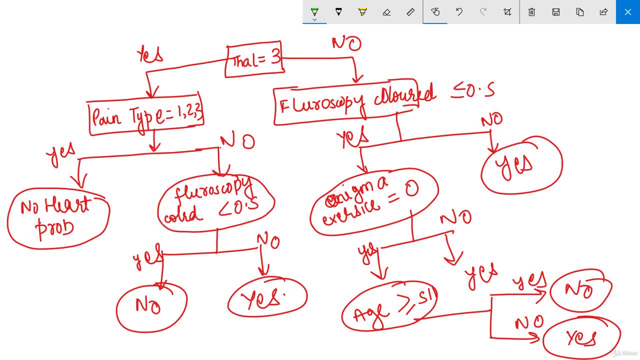 tree. you can see if what is happening here is if something known as thal is equals to three, like your doctor will check the reports and your thal is equal to three and if it is three he'll say yes. so he'll check the pain type. if pain type is from one, two or three. 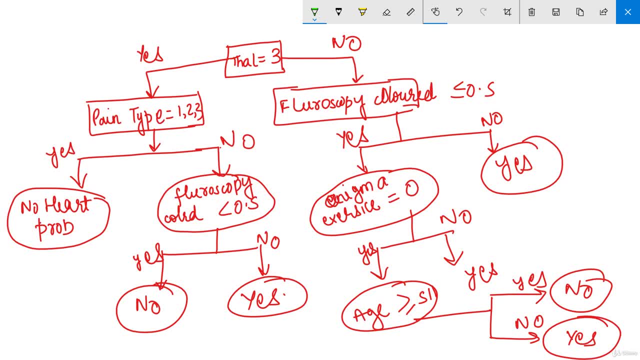 the level of pain is one, two or three. yes, so there is no heart problem. if the level is more than three, like it's not one, two, three, it's more than so. no, then he'll go for fluoroscopy, fluoroscopy colored, and it is less than 0.5, and if it comes, value as 0.5. so, yes, like fluoroscopy. 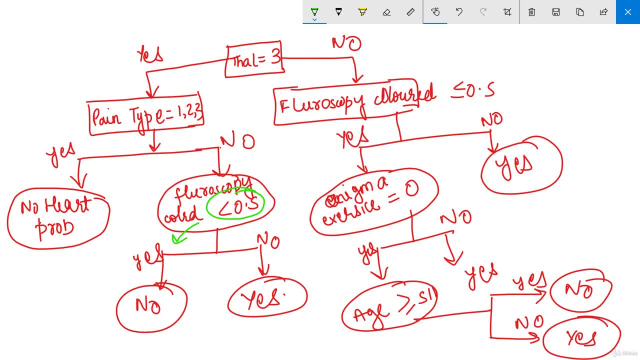 colored comes to less than 0.5, so yes, so there is no heart disease. and if it comes more than 0.5, so there is a heart disease. and if thal is not three- like the value is not three may be less than or greater than three- so a doctor will ask you to go for fluoroscopy colored and it should. 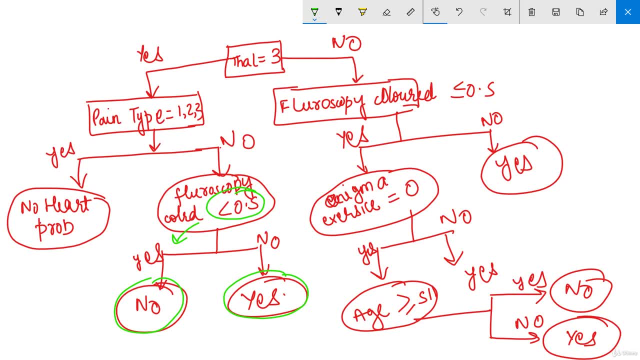 be less than or equals to 0.5. if it is less than or equals to 0.5, he will ask you to do enigma exercise. and if it comes to zero, and if your age is 51, you have a heart disease greater than 51. and if it comes, if it doesn't come to zero, so yes, you have a heart disease. 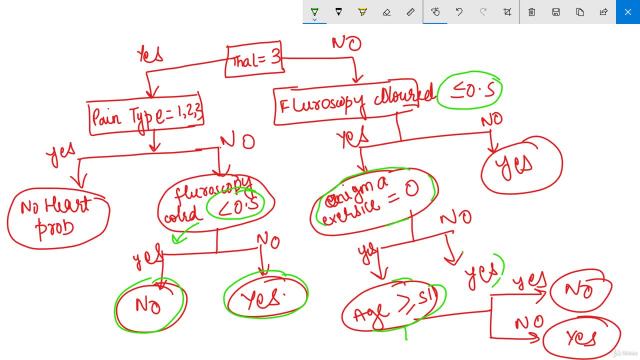 something like that. so, guys, I don't know what are the medical terms here, but this is a very good example of decision tree. right, look, just ignore the terms and look at the tree. you, this is your root, this is your root note, this is your root note and this here you will be providing. 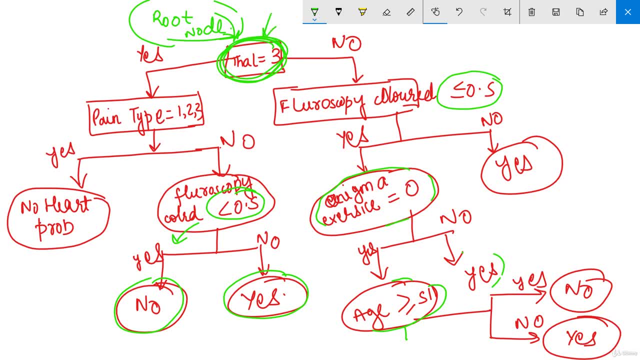 your testing data. your testing data will be entered here and everything will change, and this is how decision tree grows and everything is taken care here. I hope everything is clear up to this right, so you don't have to make a note of this if you are cleared with the decision tree in your mind. so, basically, this is how we come up. 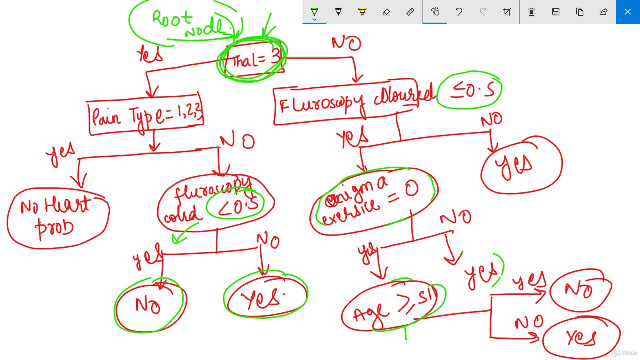 to a final decision with the help of decision tree. so, and and those who are from like, uh, coding background, any coding background, you must be, you must, you can compare it to your if else code in any like Java, if else, like, if it is yes, go here, else go here, if else. so it is very. 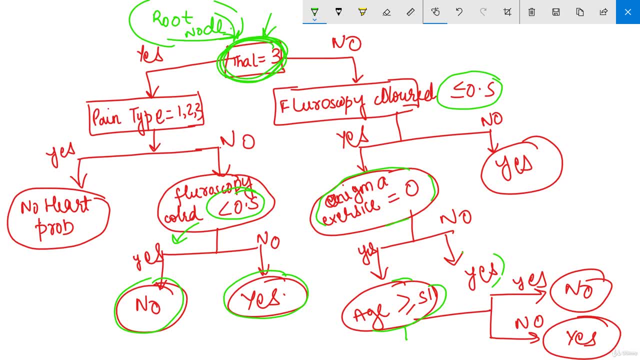 similar to your, if else coding right, those who can compare with that. all right, so I hope you are clear with the decision tree basic model structure, how it has looked, how it looks like. if you want, I can give you n number of examples like this, but I hope three examples which I have explained from basics of the room. then 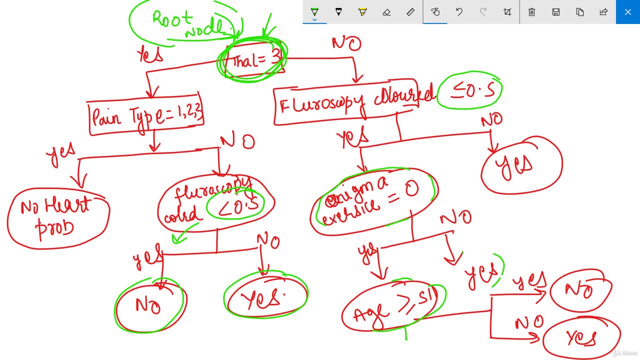 easy doctor example, and then highest with all the medical terms. decision trees can be more than bigger than this. branches can be bigger than this as well, so stay tuned. you will be facing in a coding part, like maybe after two lectures. you will see a coding video where I have worked. 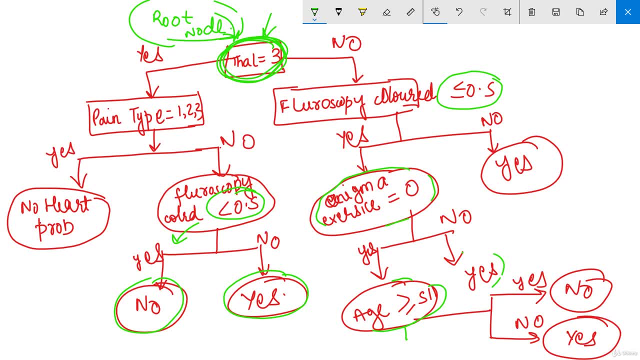 on a project of decision tree. it's a big project where each and everything is explained. I have explained so slowly and nicely that you will having no doubt. but whatever I teach before the coding, the theoretical part is getting Ur時. I know what to answer something not just super practical, but what more I teach before the coding? the theoretical part is important, but whatever I teach before the coding, the theoretical part is important and that will definitely affect the progress in future beginning. the third is 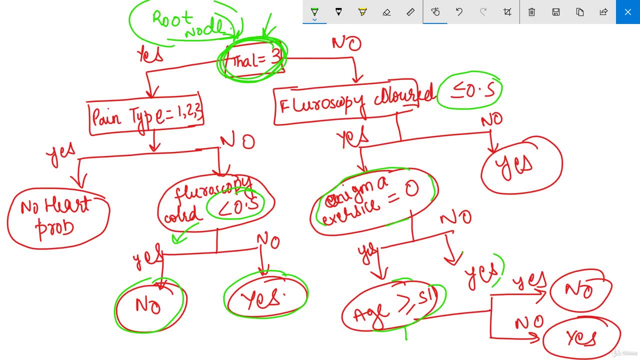 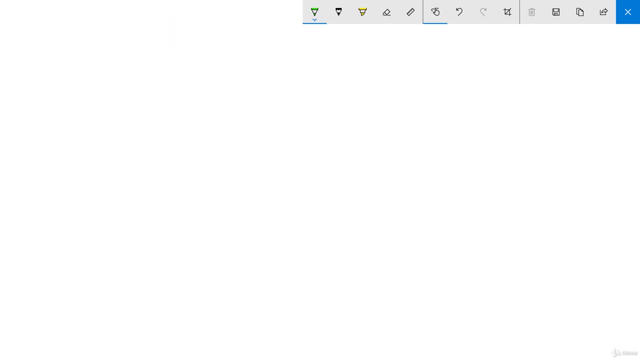 important. so you have to make note, make a note in your, into your mind, all right. so I hope, if you are clear up to this, I will jump to the next point, which is also the important point in the decision tree, which is your homogeneity. okay, so homogeneity is just how to. 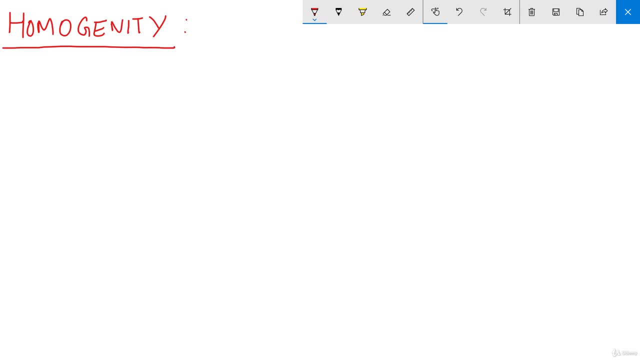 decide and divide which leaf will have what and how much like if this is leaf. so so, after dividing like which leaves like, how to divide, like what are the number of leaves possible and what values to be like stored here and how much values to be stored here, everything comes under homogeneity that you will be seen here. 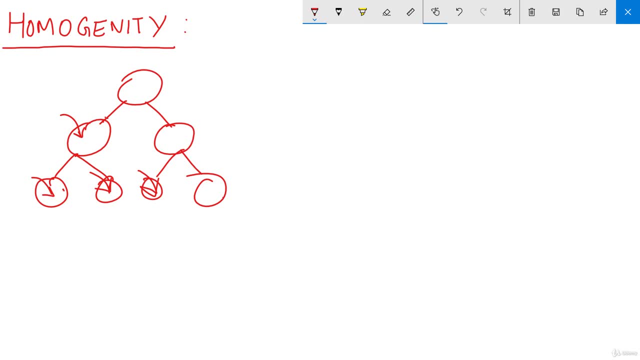 okay. so if I want to give an example here, I can give, let's say, BP blood pressure is greater than 150. if blood pressure 1 get is 150. so age less than 70, a greater than 70. so this value likes like age and the value less than 70 and 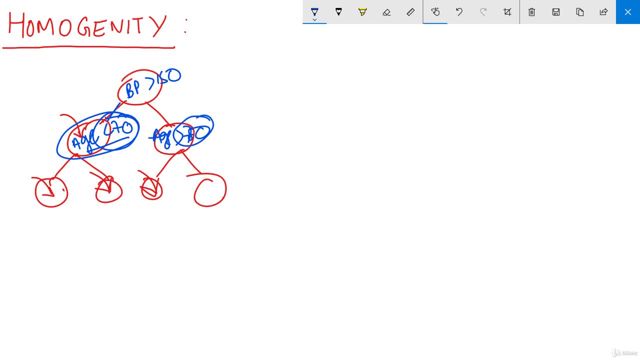 divided by 1.. So if I am dividing into two parts- less than 70 or greater than 70, or maybe between 30 to 40, 40 to 50, or there is a third left- 70 to 90, this is homogeneity, this. 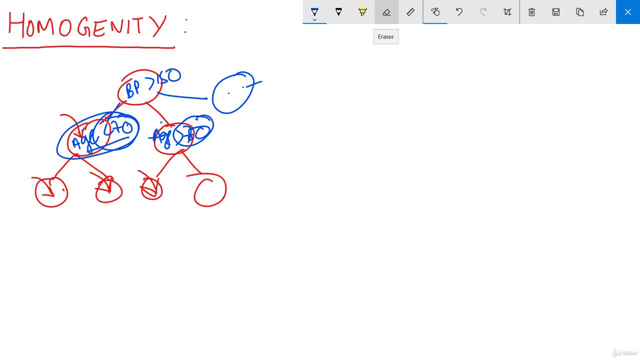 we will be studying in under homogeneity how to decide and divide it. so here let me, let me just open one more thing here. all right, so can I erase this or I'll do it here? okay, so there is a rule in homogeneity. there is a rule- or you can even say a pattern patent- that has to be. 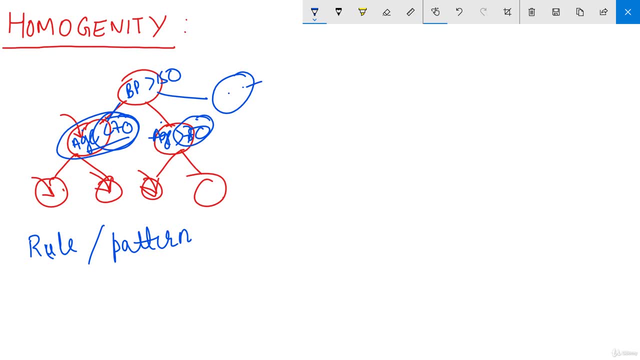 followed for accurate results, like the results should be accurate here, and this is the after: getting accurate results by following some rules. this, everything is known as homogeneity. this concept, basically the concept is known as homogeneity. now to explain you by given example, which i am very good at. so let's say we have a root here and it is further divided into two parts. 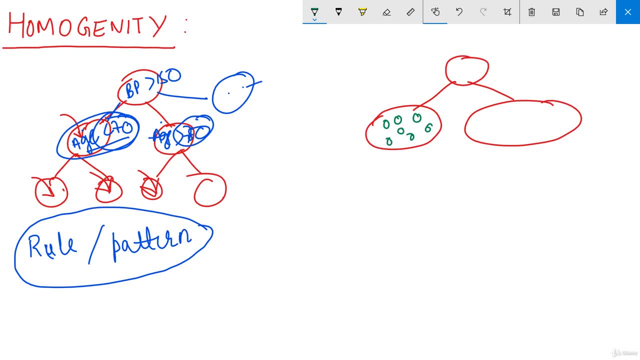 it has some circles and it has some crosses. okay, so guys, uh, you can see, these are in one leaf they're only circles and in another leaf they're only crosses. so here we can say: homogeneity equals to one, which is your maximum homogeneity? this is. 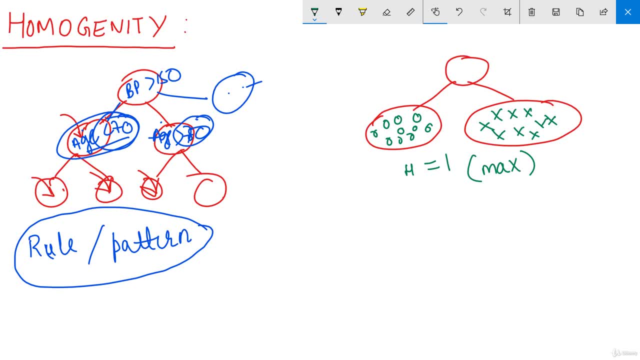 one, so like you can. this is not possible in real life. it's almost in real world. it is almost impossible to get homogeneity equals to one. but uh, like for for perfect result, we try to get h value very close to one, so like this is very in real world scenarios or data sets which will 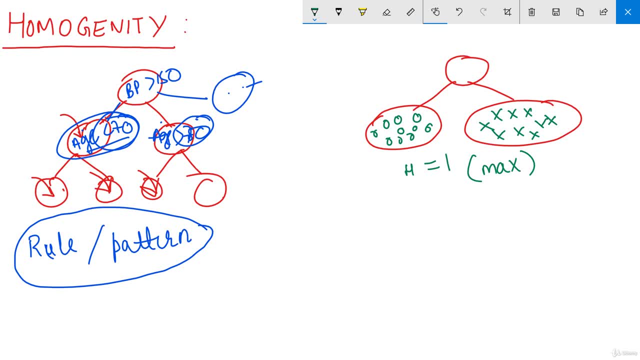 we will be doing. homogeneity equals to one is almost not equal, so one is max here, like almost not possible here. so you can also say: this is your: if h equals to one, this is your best homogeneity. this homogeneity, you can call it as best homogeneity. okay, so all right. so this is this. 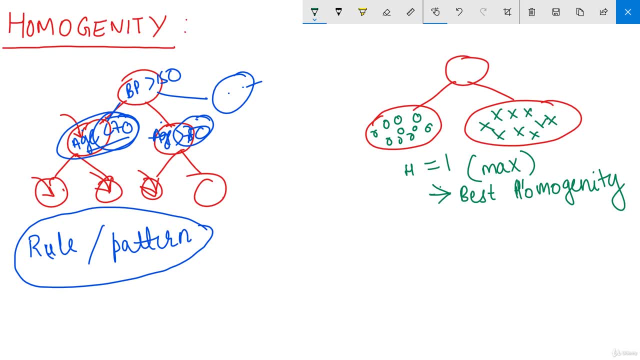 i must show you the real world example, how real world homogeneity looks like. all right, so in real world, if i want to take the same example, this can be the case. i hope you are. you are clear now what i'm trying to say. in real world, there can be some disturbances. 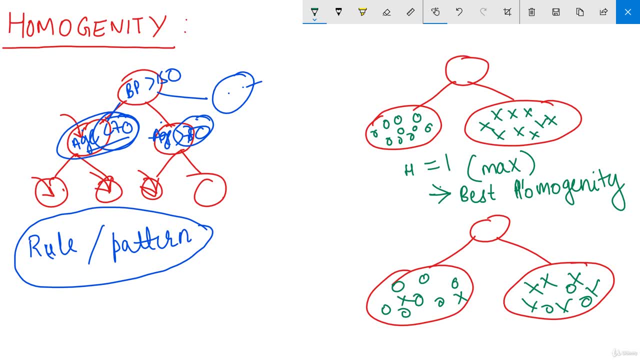 or you can say noises between the data sets which try to make, which try to make homogeneity not equals to one. here homogeneity can be approximately equals to 0.9999, which is not bad, which is also good, but this is not one, still not one, the maximum value. so we cannot say it says 100 homogeneous. 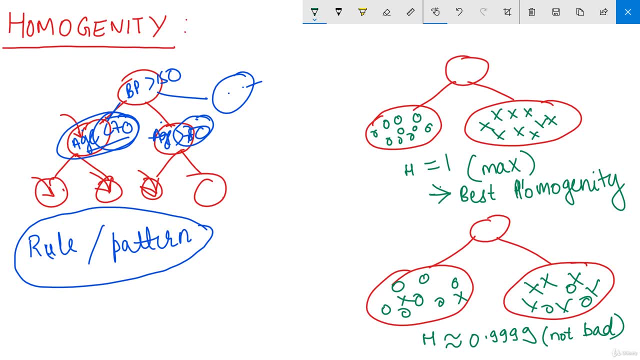 i hope you are getting it what i'm trying to say it here, and so this is not bad like. this is a very good homogeneity. if it is coming 0.9, it is very good indeed. even you will not get such homogeneity. you will be getting like homogeneity as 0.81, 0.84 or 0.9. 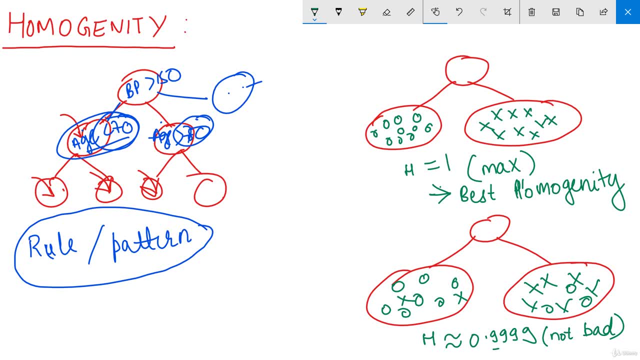 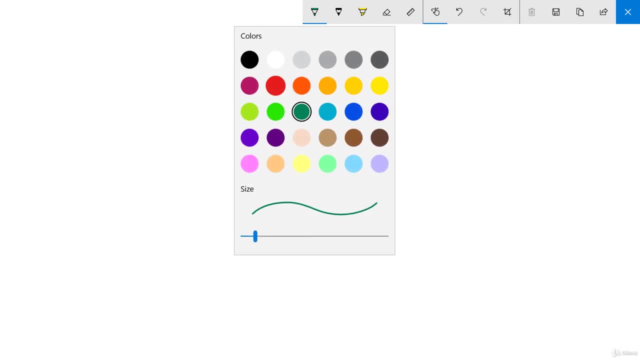 but 0.999 is a very good homogeneity, all right, so i'll just give you a example of bad homogeneity as well. let's say: this is a leaf, we have some circles. this is a very bad homogeneity, very bad homogeneity. you can say: homogeneity is 0.5 here, which is your. let's say 50 homogeneous. this is 50 homogeneous. 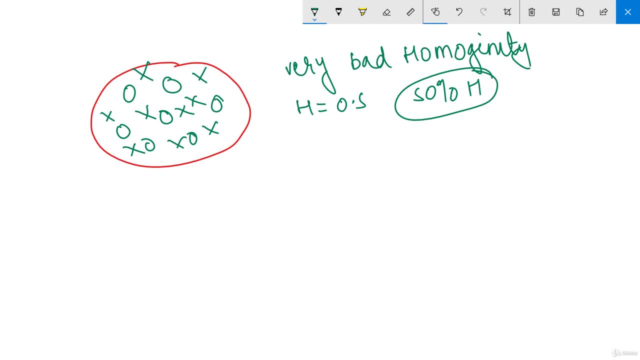 so, whatever we do, we make sure that uh, uh like, just draw a line, let's draw it here. what we have to do is if, if we have h homogeneity here in your parent node, we try to make sure that homogeneity increases when we further divide it into leaves. 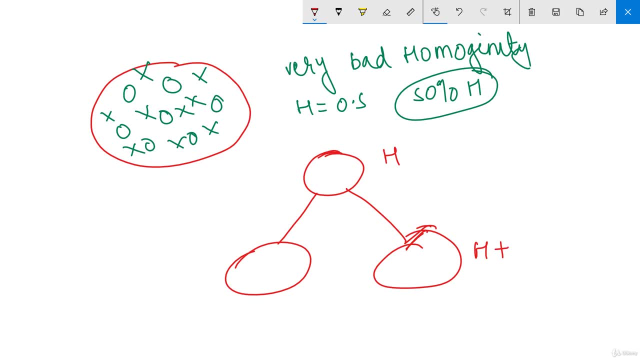 so if h is here, we expect homogeneity should increase here. and how we do that: we keep our threshold. we keep a threshold as tau, a value of tau. we keep on checking that, like we keep a, we fix a value, tau, or named as threshold, and we keep on checking that if homogeneity- what we are getting- is greater. 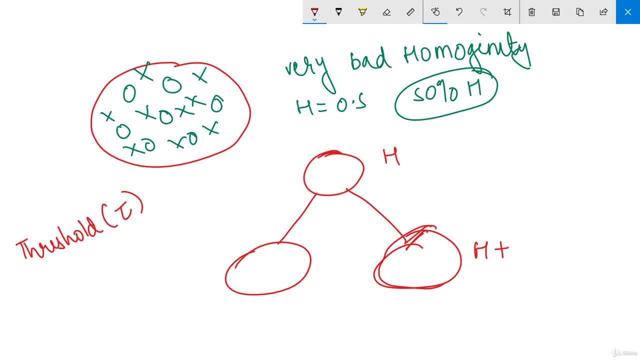 than tau. if yes, if it's getting greater than tau, we just come stop there itself and make it a leaf node and like if it is greater than tau or equals to tau, homogeneity, sorry, so we stop there itself, but if homogeneity is less than tau, 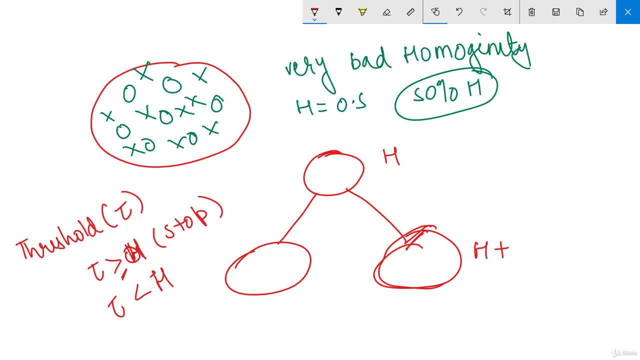 then we again keep on splitting it until your r h increases to our previous value. i hope it is clear up to this. so this is basically nothing but your whole concept behind your homogeneity. i hope this is clear, like whatever the value we have, let's say: 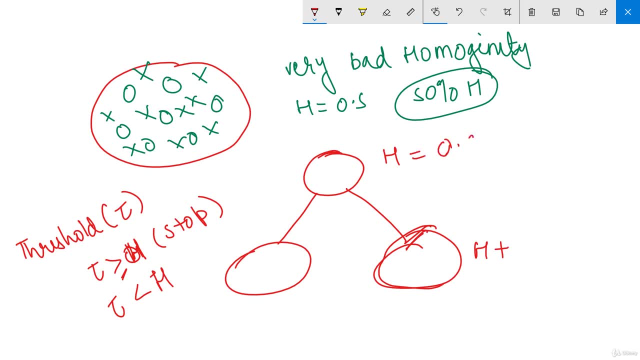 in our parent node we have homogeneity as 0.6, so we will expect in our child node we have our homogeneity is at least 0.6. homogeneity is greater than 0.6, not even equals to. we expect 0 point, maybe 0.62, 6 or 0.69 or 0.72. 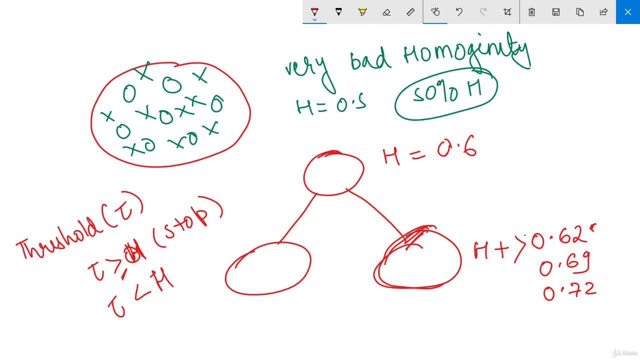 we expect a little higher homogeneity than our previous one. that's what i'm trying to say and that's what how it happens. right, clear up to this and guys trust me, like, if you're not getting it in, to this theoretical concept, even i'm trying to explain i'll. i'm going very slow in giving you. 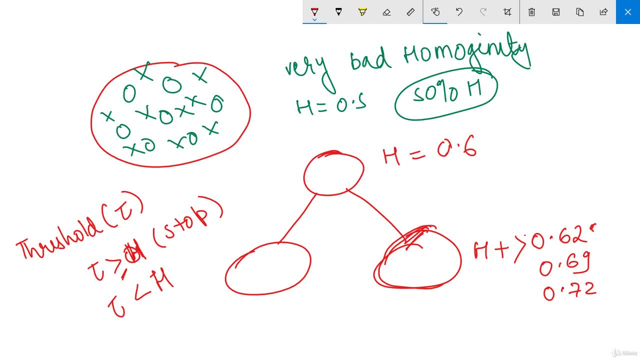 examples. but when, after this these lectures of uh, of decision tree, there will be a project, and in the project, when you will be doing practicals, like hands-on, everything will be completely cleared into your mind, okay. so this is just the basic of what we will be doing in practicals, okay. 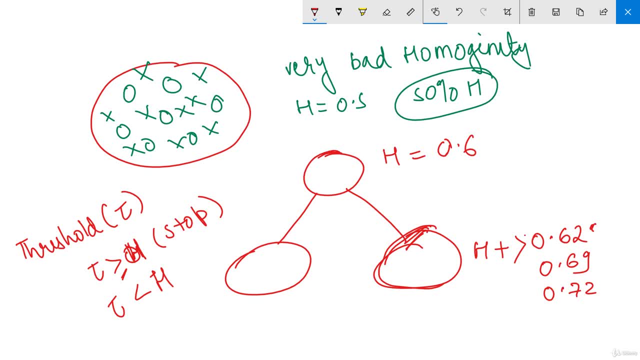 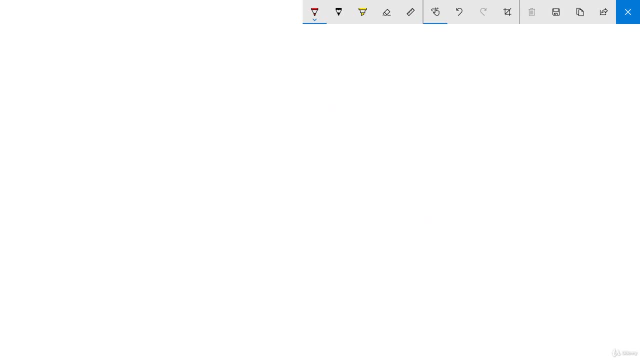 so i hope you have written this, so i'll just erase this. now let me give you another example- not example, another concept, which is your guinea index. this is also important, i can say, like entire decision tree is very important. so, whatever the uh topics will be covering, i will be covering inside it- everything will be very important. 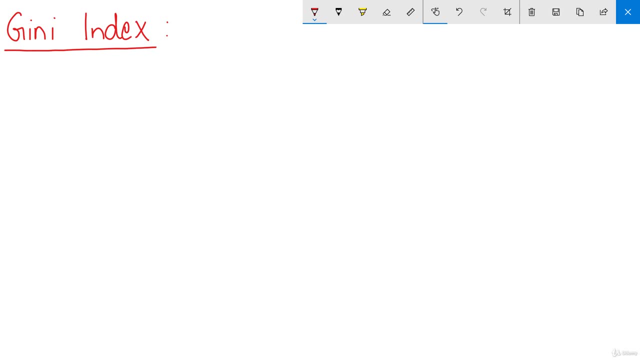 okay, so guinea index. so again, what is guinea index? guinea index is nothing, but it helps to decide what to choose choose for splitting. uh, let me write it down: it helps to decide what to choose for splitting, okay, so let me just brief you with one data set here. okay, let me just explain one data set here. guys, i won't. 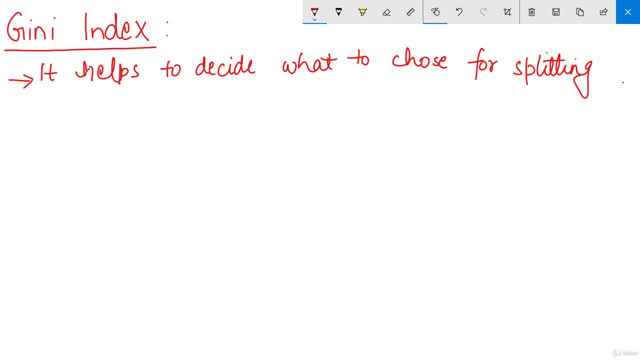 you to make this data set. whatever i'm like, i'll be drawing now. i want you to make a note because, uh, there's a continuation of that which in which i will be erasing everything from the screen, so that you can look that into your own notes and compare the values. 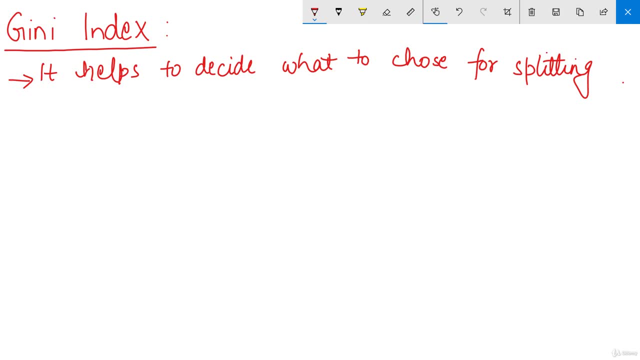 because the values will be gone if i'll erase the screen, right? so i just want you to uh ex like, first listen carefully, make a note, understand and then uh like, after pausing the video and then play it again. so let me just explain you one thing here, one concept. 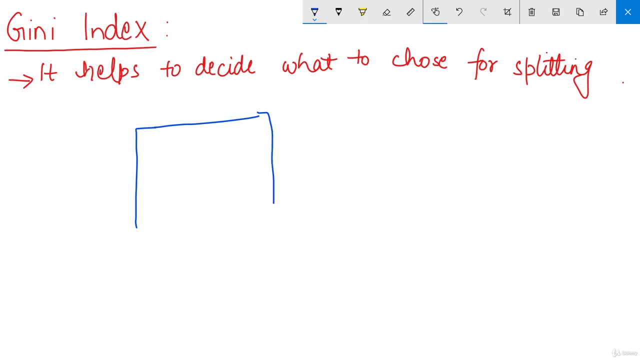 i'll just draw it first. so, yeah, i'll just like write everything. i. i would request you to, uh, you guys also write each and everything here with me. it might look complicated right now, but it is not at all complicated, trust me. okay, so this is what i want to explain. so this is nothing but. 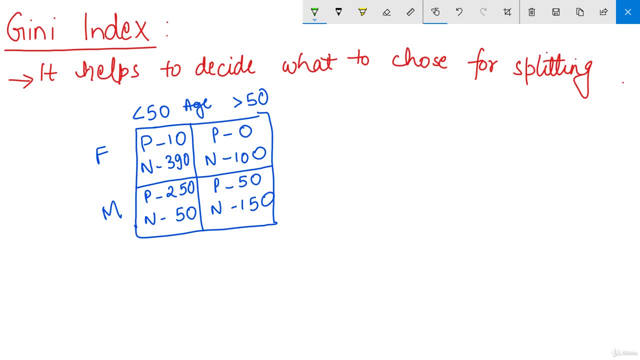 a small data set which i have like shown like this, in which this part, um, the left part from this line, green line, the left part is your, uh, your people less than age 50, and right side are the people greater than each of 50, and the top one are female and the bottom one are male. so this is nothing, but this is a survey. 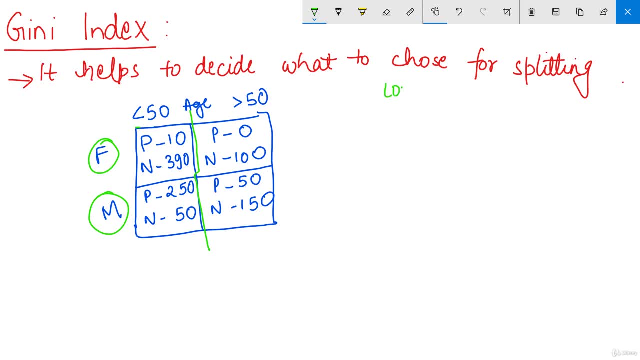 who loves to play football. Like, I'll just write: loves to play football. This is a survey on that. Alright, so less than 50 age, like if the person is less than 50 years of age and gender is female. so there are 10. who loves to like positive results. 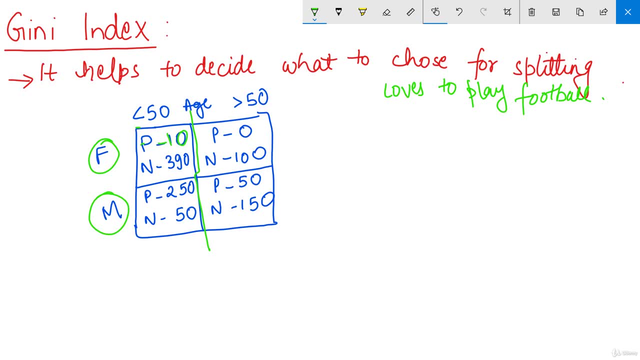 P is positive and S is negative. So 10 loves to play football, 10 females love to play football less than age 50, and 390 does not love to play football at all. And greater than 50, 0 females like to play football and 100 they simply don't play. 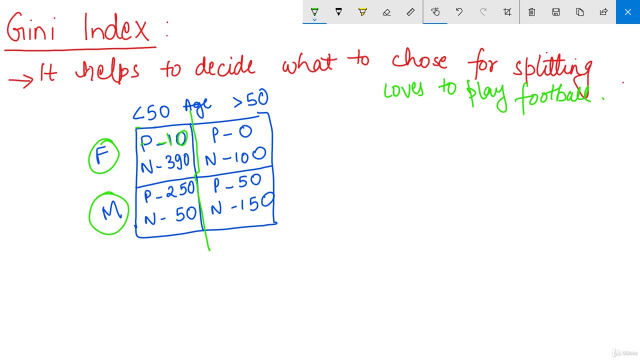 So nobody likes to play, and okay. So similarly, with male, 250 love to play football And 50 does not love to play football. And at the greater than 50 age: wow, 50 people still plays football and 150 don't play football. 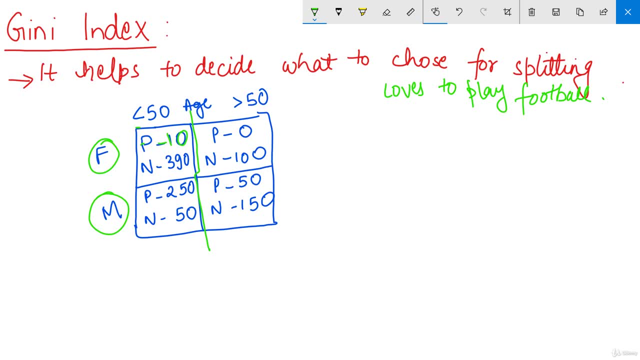 So this is what our data set is looking like. I hope now you are clear, but this is not that complicated. So if I want to split it on the basis of gender, On gender, let's take females first. Females: 10 females play football. 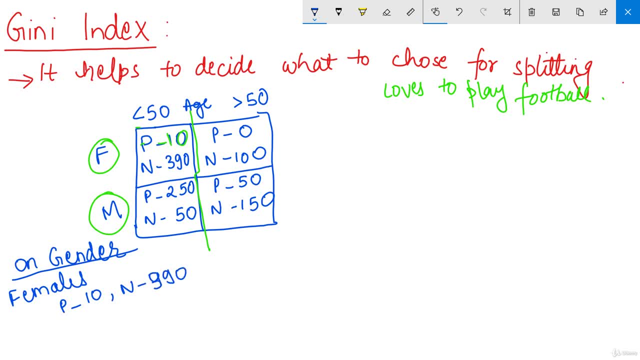 490,. I'm sorry, 390 doesn't play football. No, no, Yeah, it's 490.. Sorry, 490.. Yes, because We are taking on the basis of gender, so we'll take entire thing, not age on age. 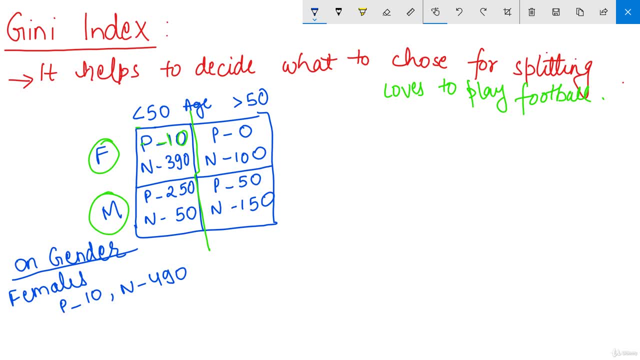 We will taking the this part only. So 490 doesn't play. So total we have 500. for males who love to play football is 300 in total. You can see in males you can see they are 300 in total- who loves to play football. 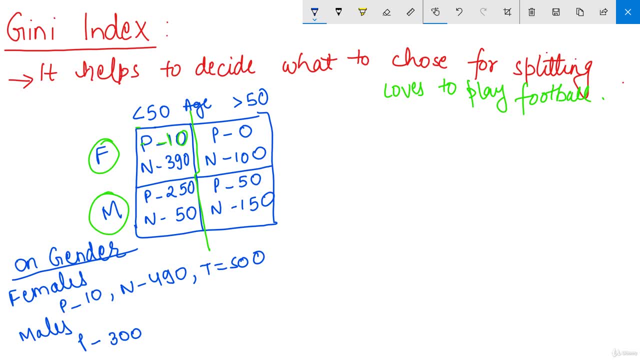 Right. So like 250 plus 50, 300 and 200 doesn't play football, So your total is again 500.. This is on the basis of gender. I guys, I want you to make a note of all this because the next step- like I have a note of all these things, but I will see from that and I'll do the rest- calculation. 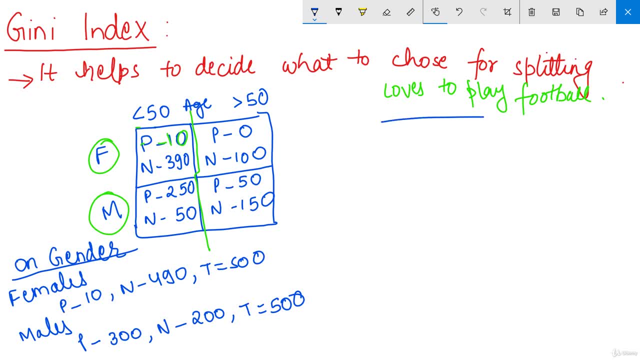 But you should have a note as well to understand what I'm trying to explain here. So this is on the basis of gender, and the basis of gender we ignore age. now, on basis of age, here we'll ignore the gender. Okay, so if the age is greater than 50, age is greater than 50, 50 people plays football, 250 doesn't play football. 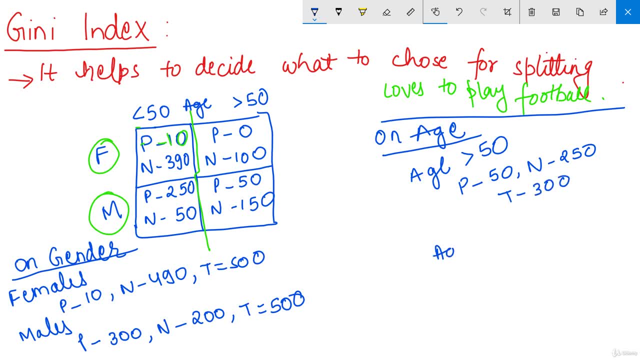 So total is 300. If the age is less than 50, and 250 plus 10, 6, 260,. 260 plays football, 440 doesn't play football, and the total we are getting is 700 here. 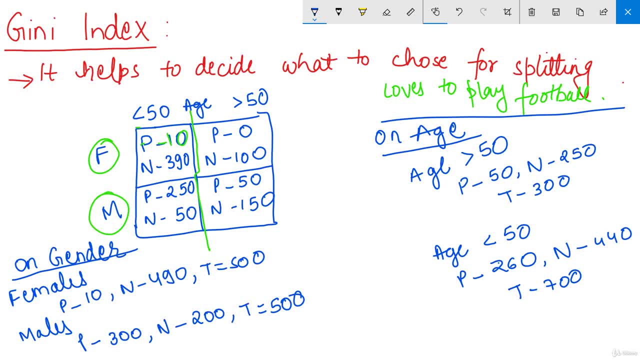 Alright. so, guys, I want you to make a note of all this, because I'm going to rub this, and then I'll explain one concept here: a formula on the basis of Gini index, Which is also the project is completely based on Gini index, which I will be working on. 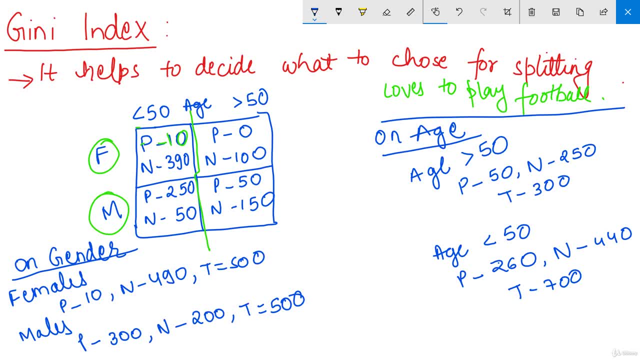 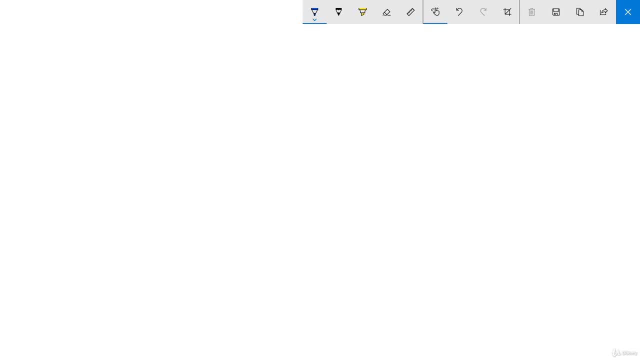 So I want you to make a note of all this. Okay, so I'll just erase, you can pause it. Okay, so now let's take the probabilities. Probabilities of let's female is obviously 1 by 2 because male and female, so probability is 1 by 2.. 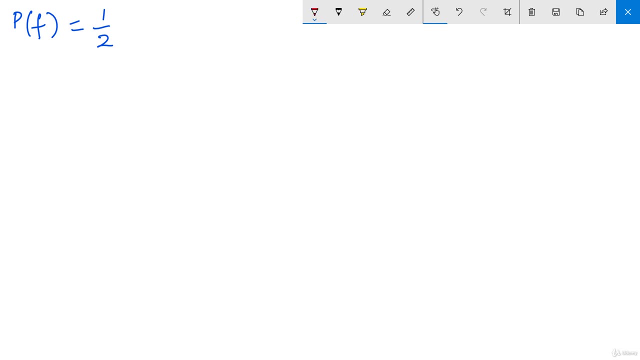 And how to find the Gini index. So, Gini, there is a formula for Gini index which is from I1 to K, probability whole square. So what we do here is we look at the probabilities and square them up, nothing much. 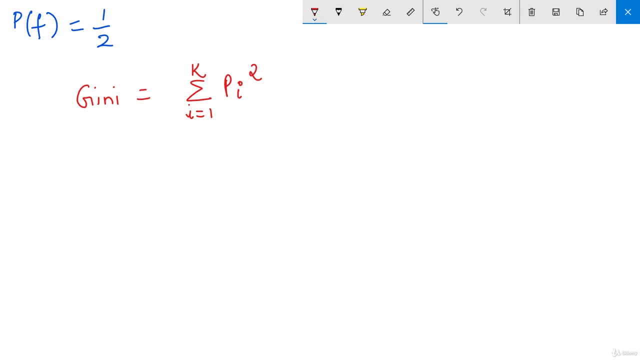 So I'll explain you how we split: now on the basis of Gini index, or that, too, on the basis of gender. Now on gender, splitting on gender On the basis of gender. let's split and put this into the formula. So Gini is probability, is 1 by 2 for female. 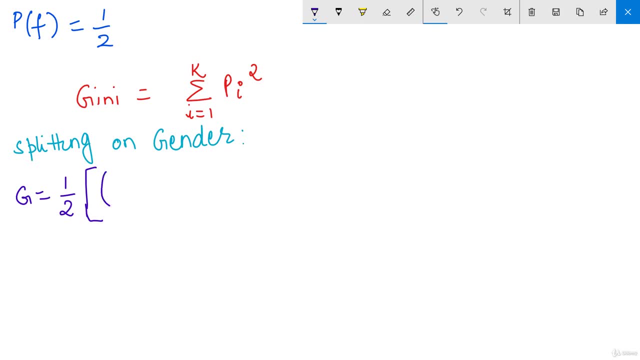 and 1 by 50. I hope now you understand why I was 1 by 50. you have to find the probability there from the back. that is why I'm say I'm saying that you have to have all the nodes in front of you. so 49 by 2. this is we are talking about. 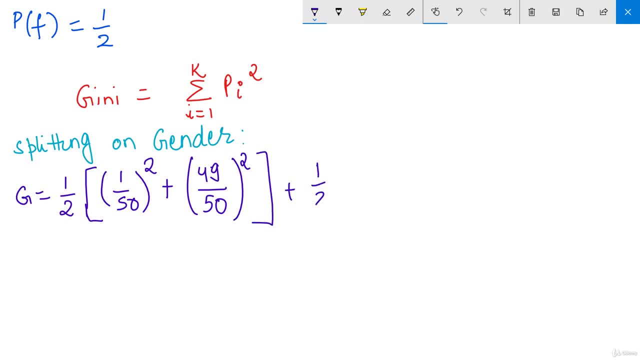 females first and then males. probability is 50: 3 by 5. if you solve this, you'll get a value of 0.74 on. this is splitting on the basis of gender. now if I want to split on the basis of age, it will somewhat look like 0.7 to 60 upon 700 plus 440 upon 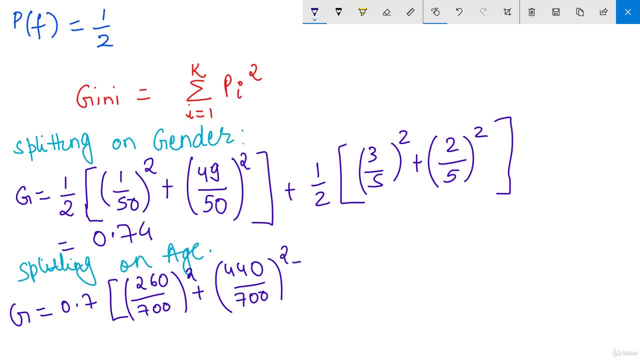 700 plus 0.7, so it will be 0.3 depending upon the AO number. so here creating the only one for yourrah probability is 1. together it makes 1. probability is always 1. so D by 300, 50 by. 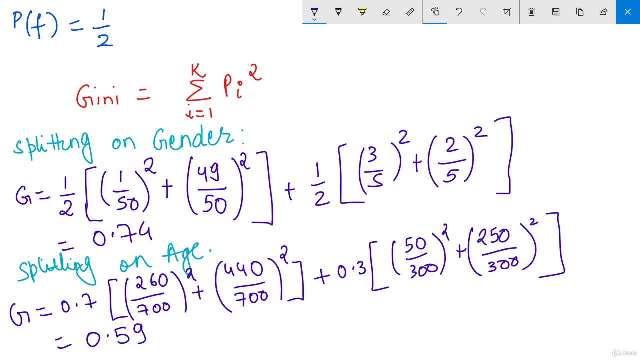 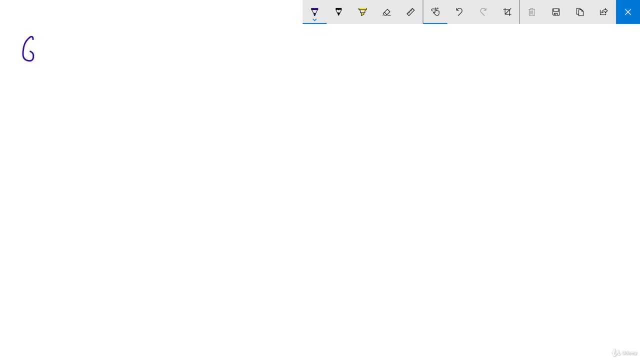 you will be getting a value as 0.59. okay, so here you can now here. I think I should erase this page again. so guinea index on the basis of gender: I'm getting as 0.74, and guinea index on the basis of age: I'm getting as 0.59. so, guys, this is. 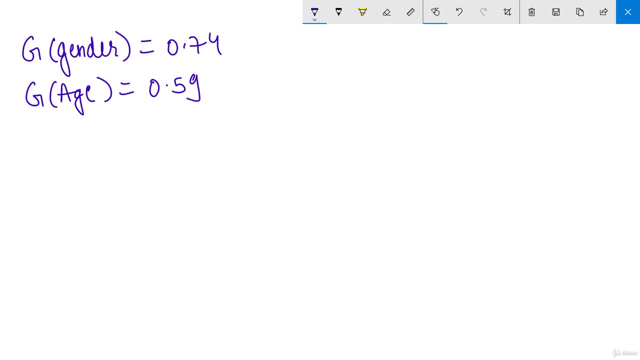 how you calculate your guinea index. and after calculating your guinea index, you just compare which one is greater, closer to one, and whatever the value is, obviously you will take that. so here we will be taking, like taking G, gender as my guinea index and we will be splitting on the basis of gender only. 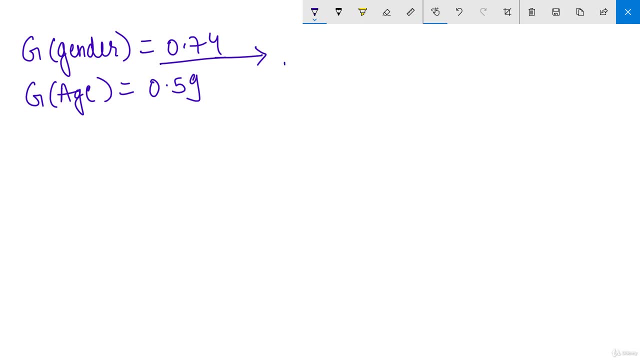 and if you see the data set, what I have written, what I've shown you, I think I can go back. make sure, no, no, take a lot of time. so, like it is obvious, like we will be splitting on the basis of gender only, right, so age will not matter gender. 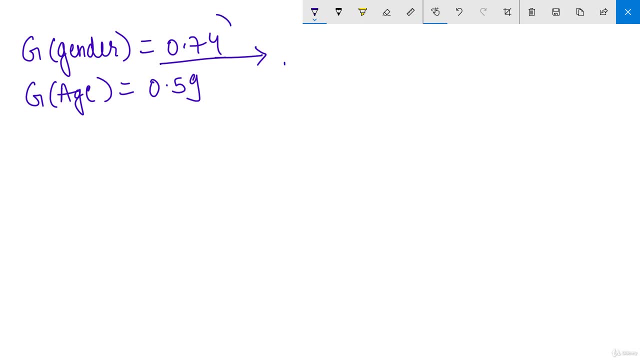 will matter in this case, in our example. so this is how we will be doing guinea index splitting here. so it is easy, right? not that difficult. we just know a simple of probability and you just have to find everything out there. so whatever the value is greater, you have to take that. 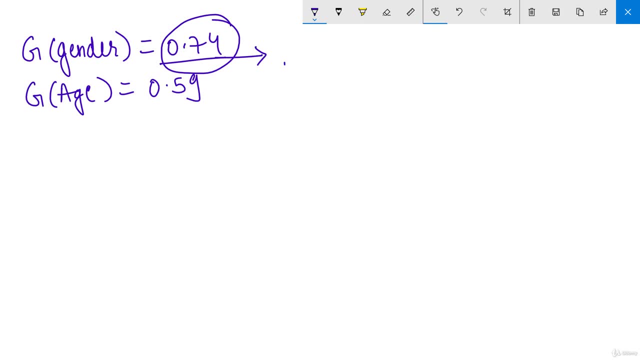 and you have to split according to that. okay, all right. so, guys, in next video you will be seeing another concept, but first I will start and end this video. so in this video I'll be talking about LFYT traditions in general and I'll tell you what LFI attributes are once more, what all the values of lutton are. OK, those are theiałem countries and something that is useful to you is one of the hobbies, really good. OK, let me see what some heavy bit terms and put it on here. so first, this is a step that I use next here, without food and snack for the beginning part. 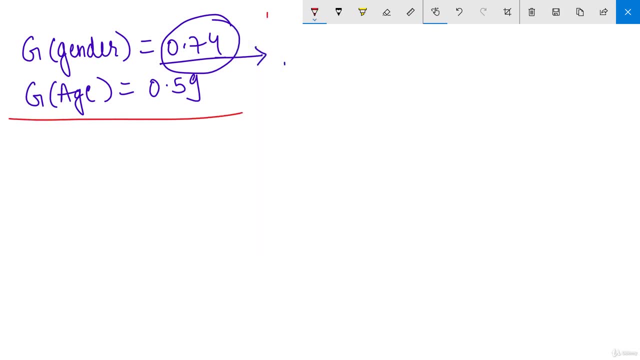 concept: same thing, but in different way. it will be your information gain, which in which we will be using a lot of entropy terms, don't get afraid. very easy, very, very easy, and a lot of things like this entropy, and you will see like it is completely opposite to your guinea index. like not opposite, you can say inversely. 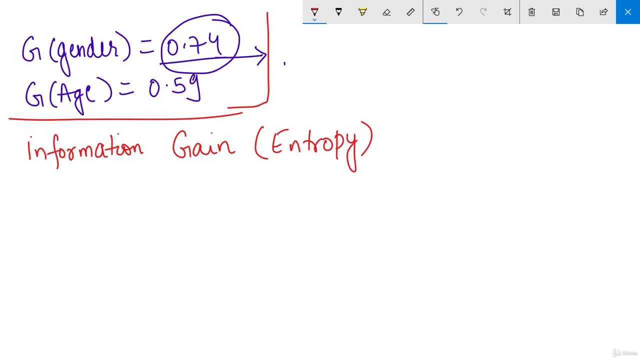 proportional to your guinea index and everything you will be seeing in our next lecture. so- and it is very important as well as interesting as well- information gain part. so I hope it is a guinea index part. the decision tree part up to guinea index is cleared into your mind and if it is not, watch this video. 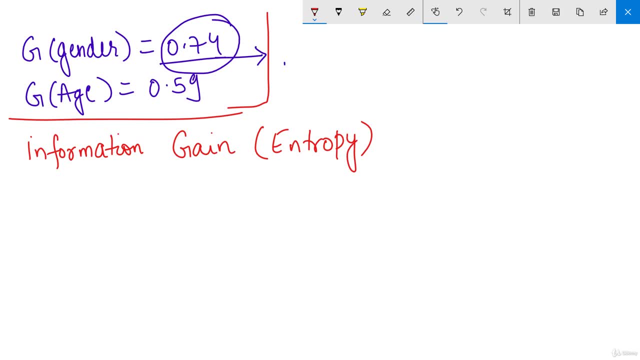 again and again, two, three times, five times, ten times, but make sure it is clear into your mind and then move forward to your information gain. nothing is difficult like. if you think it is something is getting difficult, even watch it again and again. everything will be cleared. all right, so I'll just end this lecture here and you can move.